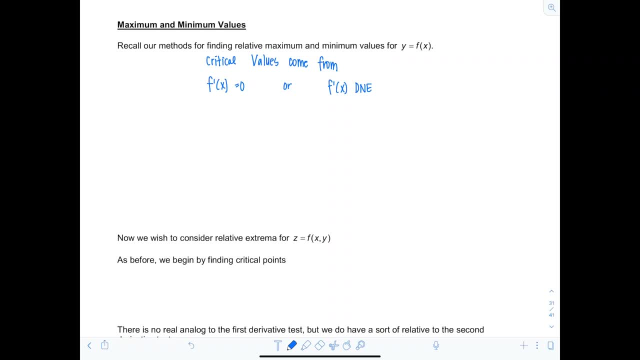 your critical value was a relative max or min. you had two options. You could either apply the first derivative test And then in that case you would make your little number line representing the values of f, prime of x, And then you list your critical values on the number line. 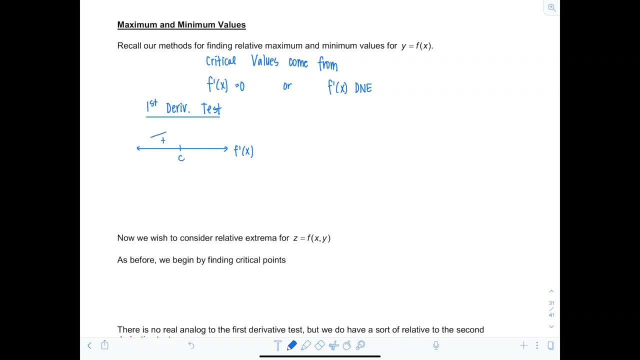 And then remember if it went from increasing, if the derivative was positive, and then to decreasing on the other side of the critical value. then you knew, at your critical value, your function achieved a relative max And the other scenario would be again making the number line. 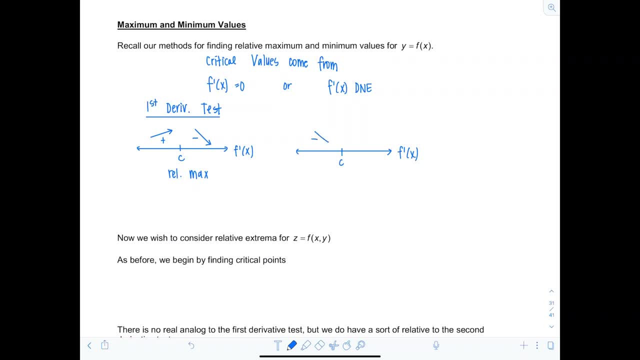 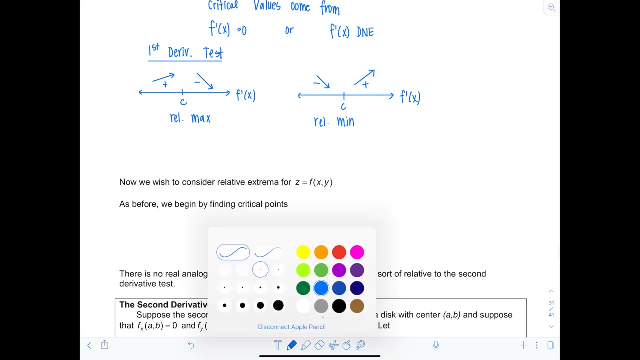 for f, prime of x, you put your critical value. If it went from decreasing, if the derivative was negative and then it switched to being positive, so the function was increasing, then you knew you achieved a relative min at the critical value. Another nice option which usually you use in: 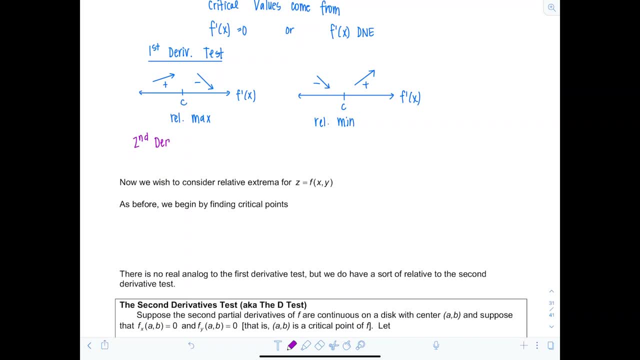 optimization problems is the second derivative test And that's still to test for local extrema. Remember, if you have a derivative test you have to test for local extrema. Remember, you look at the value of f double prime at the critical value And if it comes out to be, 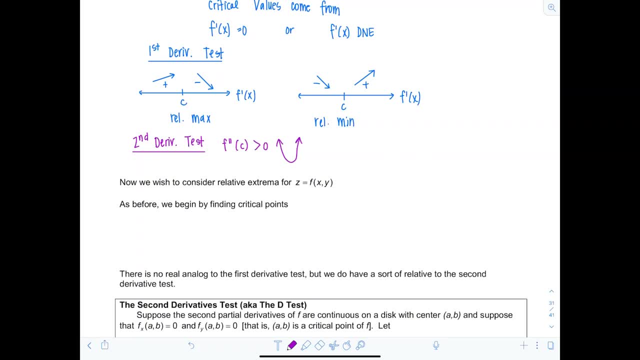 positive. well, that tells you that your function is concave up at that point. But since you know that c is a critical value, then it must be a relative min. You know that the derivative is either zero or doesn't exist there, So you know it's going to be at the minimum, Or other case. 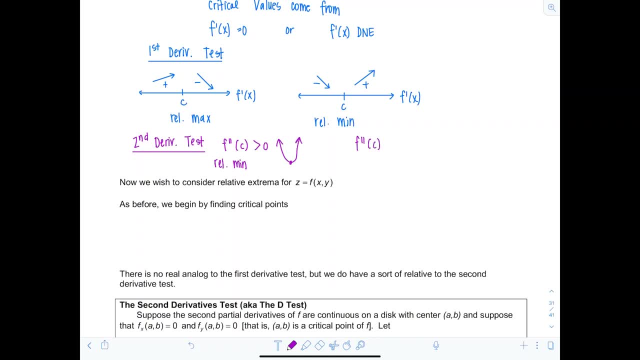 f, double prime of c would be less than zero. Well, what would that tell us about the concavity? Then the graph? the graph would be concave down. We already know c is a critical value, which means the derivative is zero or doesn't exist. 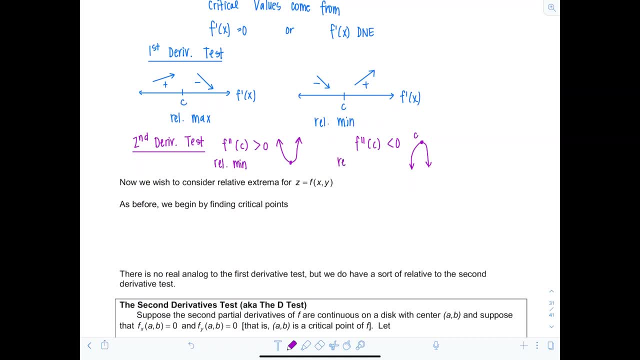 So it would have to be there And that would make your function achieve a relative max. And then remember, the last case was if the second derivative at c was equal to zero, then you had no information, Basically meaning the second derivative test was inconclusive. 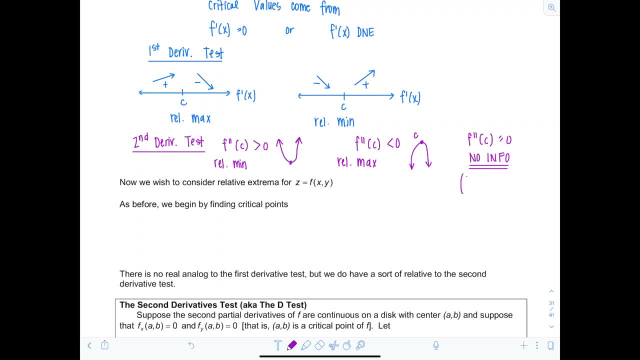 And what did you have to do? You'd have to go back and just use the first derivative test instead. So, since sometimes the second derivative test is inconclusive, usually we like to rely on the first derivative test. But, like I mentioned earlier, when you're 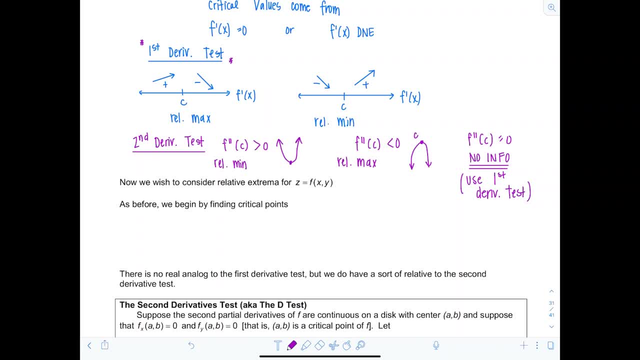 doing optimization problems. the second derivative test can be quite nice. So now we're going to see how do we apply this idea when we're looking at functions. Now we'll just focus on functions of two variables. So we'll say z is a function of x and y. 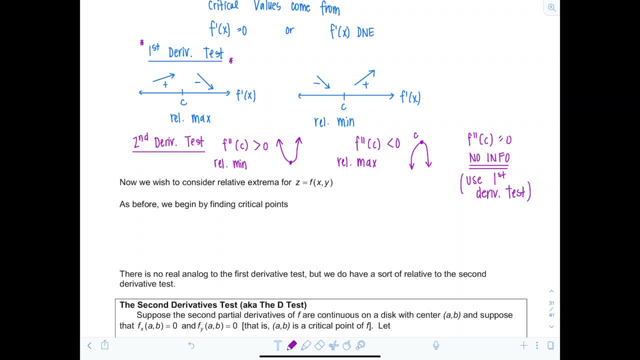 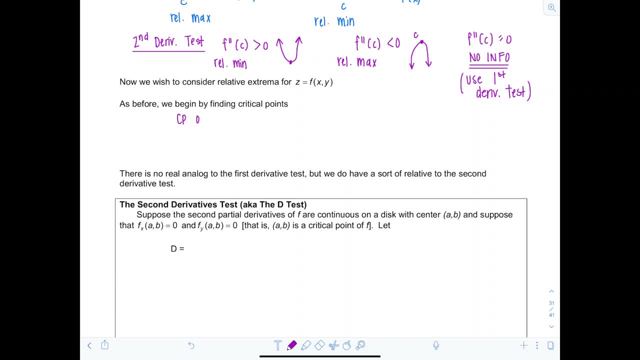 So, as before, we want to figure out where are critical points. Well, what's the criteria for critical points? It's a little bit different. So now we say that critical points occur where both your partial with respect to x and partial derivative of f with respect to y are zero. 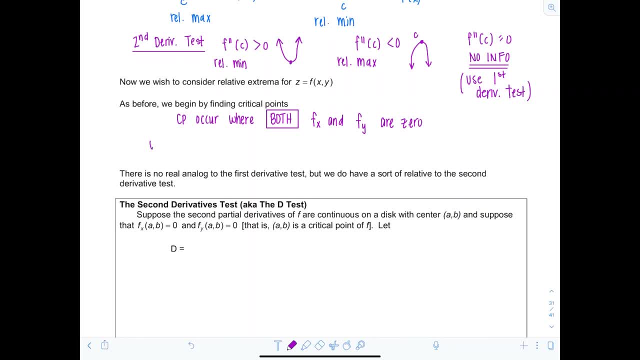 So both of them have to be zero simultaneously. Or here's the other case, Or either of them is undefined. So either the partial with respect to x or the partial with respect to y is undefined. Now there isn't really an analog to the first derivative test. There's no way that we can sort. 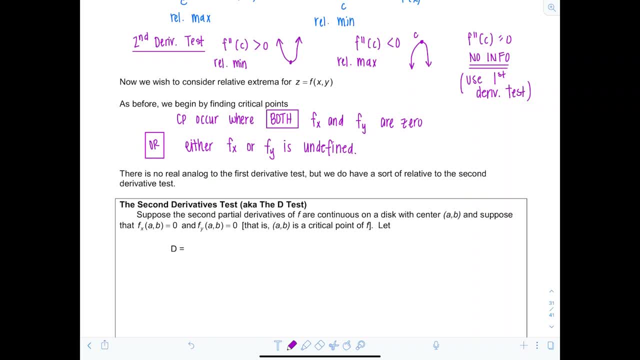 of equate that process with what we do for the second derivative test. So we're going to do for functions of several variables, But we do have something sort of similar to the second derivative test that we use, And it's called the D test. So first we have to suppose that the 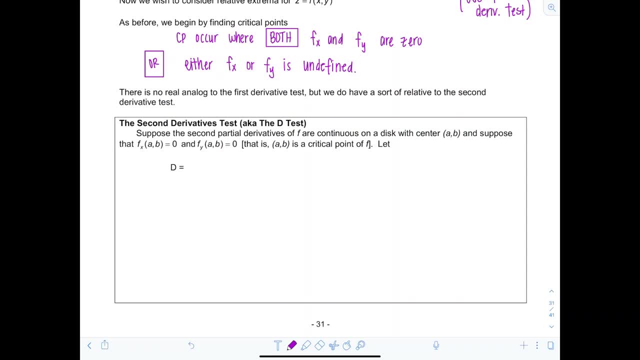 second, partial derivatives of f are continuous on a disk whose center is at ab And we're going to suppose that the partial with respect to x and y at ab are both zero, which makes ab a critical point of the function f right per the criteria listed above. 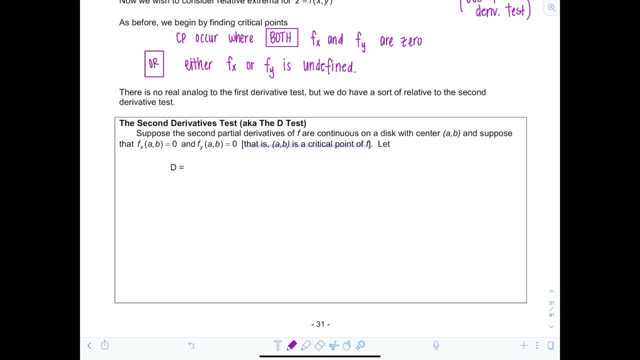 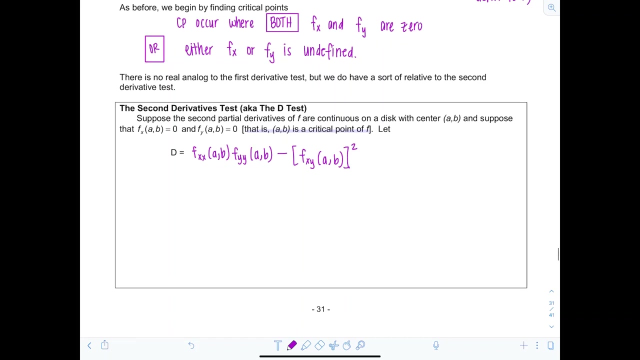 So we define this quantity capital D as follows: It's equal to the second partial with respect to x at ab times, the second partial with respect to y at ab minus, and then we have this mixed partial f sub xy at ab squared. All right, that's how we define D capital D that we use for the D test. 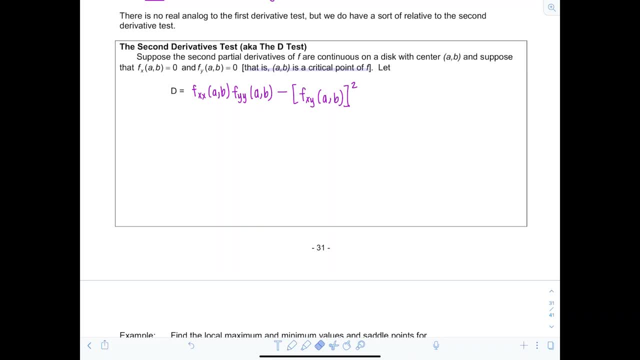 Now you're going to, once you find your critical values, what D comes out to be, and then that is your test to tell you whether or not you have a relative min, max or saddle point. So here's the criteria. Option number one: if D is greater than zero, 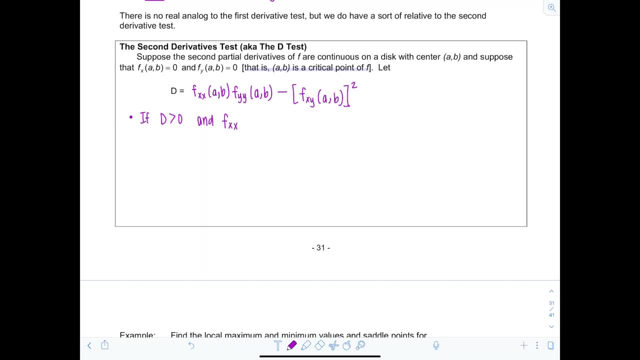 and your second partial with respect to x is also greater than zero, then f of ab is a relative min. Next option: if D is greater than zero and your second partial with respect to x is negative, then f of ab is a relative max. 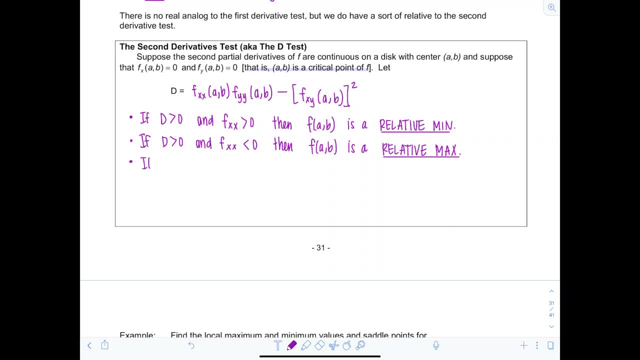 Next case, if D is less than zero, then F of AB is a saddle point. And you might remember, we've discussed the idea of a saddle point when we graphed the saddle, your hyperbolic paraboloid, And we looked at that point in the middle of it, which could be viewed as a min or a max, depending on the perspective that you're taking. 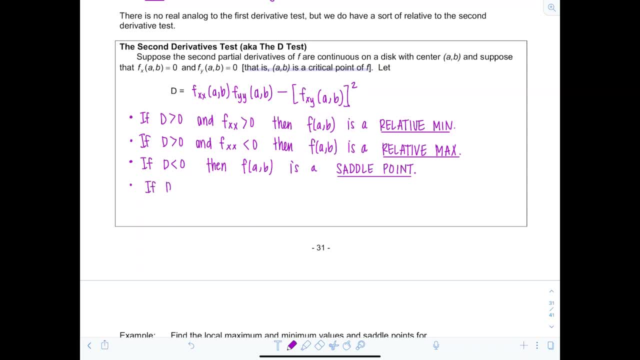 And then the last option is: if D is equal to zero. Well, what do you think, guys? Yes, it's a very sad day. Then the test provides no info. What does that mean for us? You give up? No, no, no. 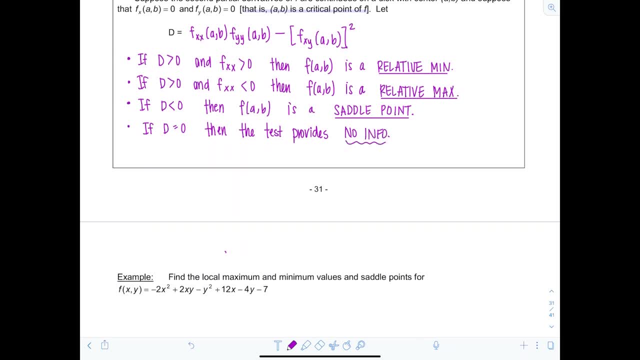 You just have to do something else. So the test is inconclusive. You have to do something else. You're still responsible to answer the question. So, don't worry, I'll show you a couple examples where this will happen to us. But we have other means in order to determine whether we have a min or a max or whatever. 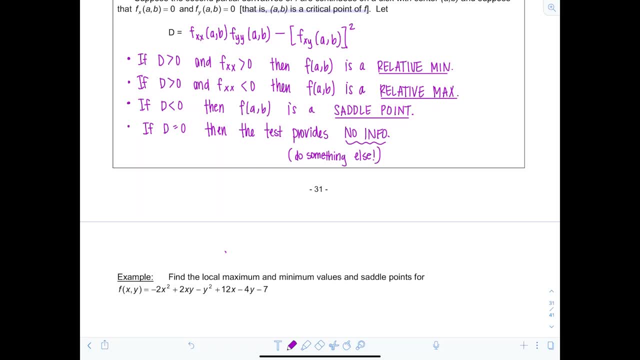 Okay, So you just have to memorize what the conditions are. The proof and explanation is a little bit much So if you want to look into that on your own time, that's fine, But we're just going to look at how to apply it now. 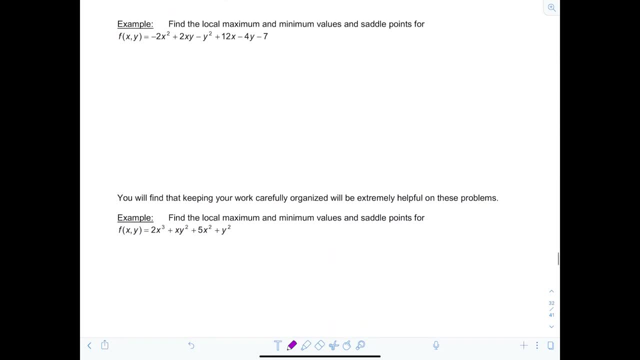 So let's find the local maximum and minimum values and saddle points for the following function. We have S of XY here, So first thing I need to do is collect my critical value. So I need to take a partial with respect to X and Y. 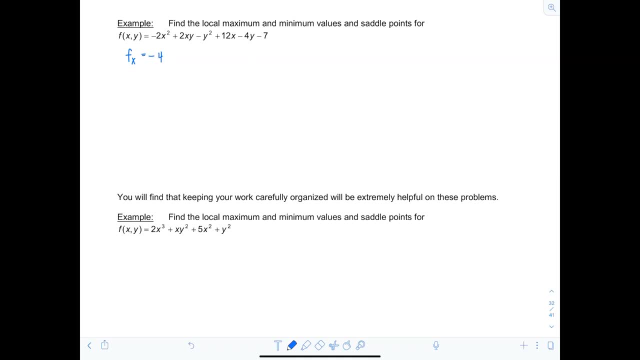 So partial with respect to X is going to be negative: 4X plus 2Y plus 12.. And then partial with respect to Y is going to be: It's going to be 2X minus 2Y minus 4.. All right, 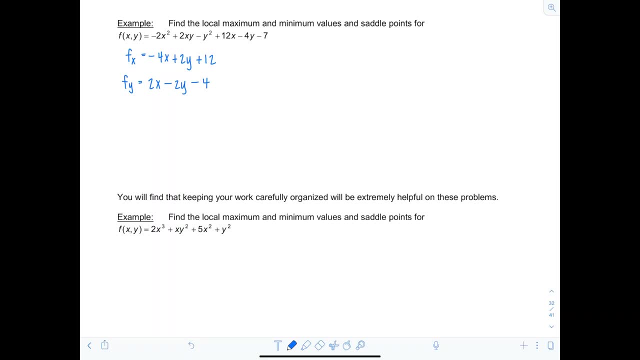 Now, while we're at it, since I'm going to apply the D test, I also need the second partial with respect to X, second partial with respect to Y, and then I need my next partial, F sub XY. So let's take another derivative, another partial derivative with respect to X here. 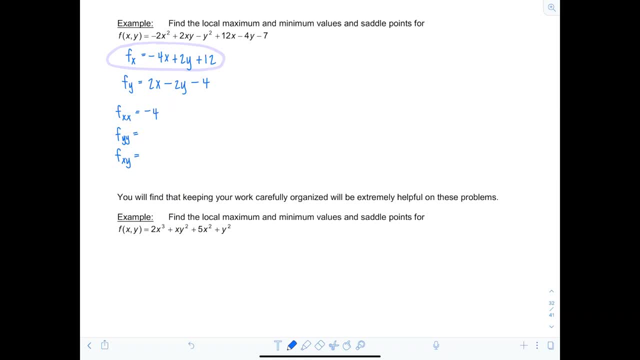 That's just going to give me the constant negative 4.. If I take another partial derivative of F sub Y, with respect to Y, I'm going to get negative 2.. And then F sub XY- that partial derivative is going to be positive 2.. 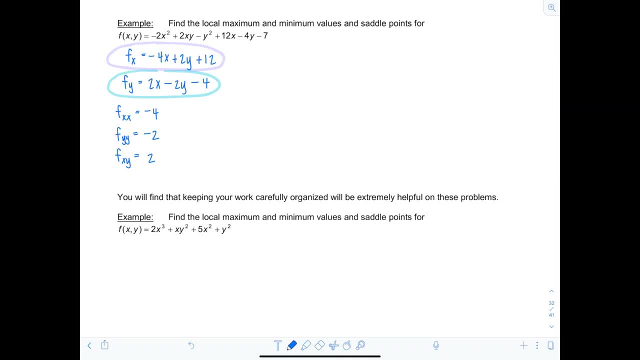 Okay, So we're done. Now let's get our critical value. So remember, I have to set each of the partial derivatives equal to 0. And then solve that system there, right? You get critical values when both partial derivatives are equal to 0.. 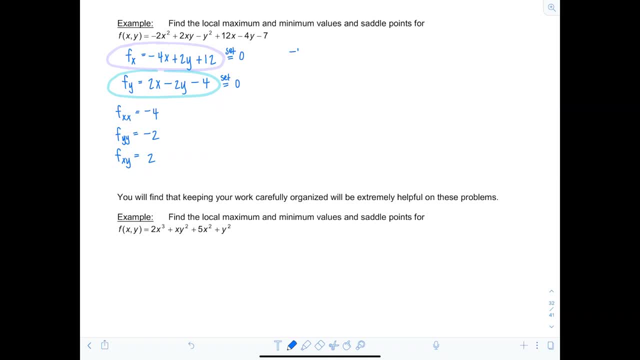 So let's see here I just have a system of linear units. So this is negative. 4X plus 2Y- I can move that over- Equals negative 12.. And then the second equation gives me 2X minus 2Y equals 4.. 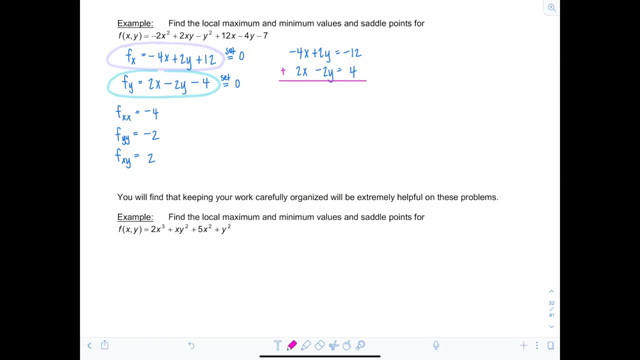 And this is just a sweet little linear system back from your algebra days. So the 2Y is going to cancel out. Now we have negative. 2X is equal to negative 8, which means X is equal to positive 4.. And then I can just 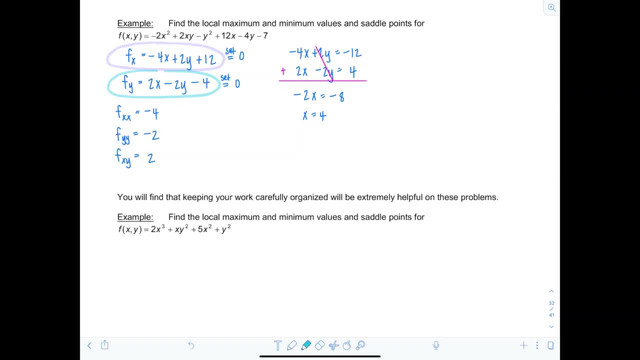 substitute that value back into either equation. So if x is 4, this is going to be 8.. Move it over to the other side. then I have negative 4, which means y is equal to 2.. Okay, so I've got a critical. 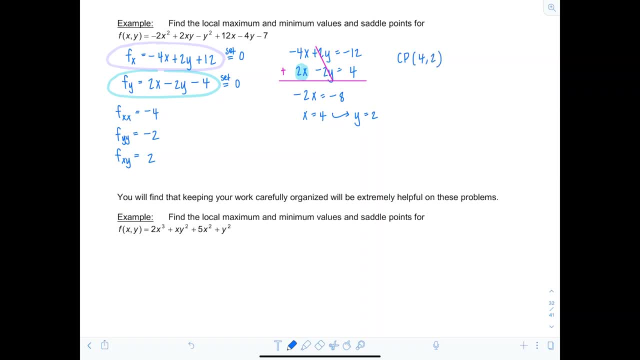 point. It's at 4, comma 2.. How exciting. Okay, now, when you have a lot of critical points, it can get a little bit messy, So I recommend organizing your info in the following way. So you're going to make a table. In this case, our table is only going to have one row, but I'll just show you what. 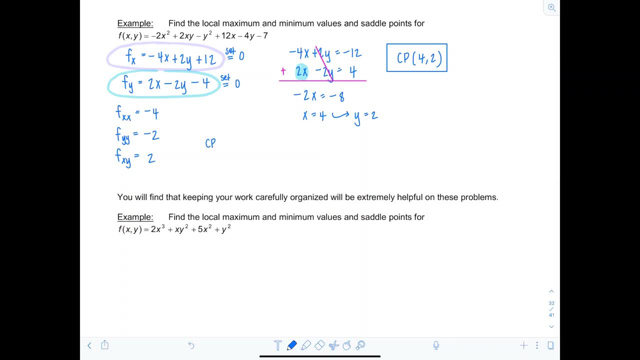 the headings are going to be on each of the columns, So list your critical points. Then you're going to list what f sub xx is. Usually it's going to be a function of x, but in this case it was just a constant. So here's our critical point. Then I want the second partial with respect to y. 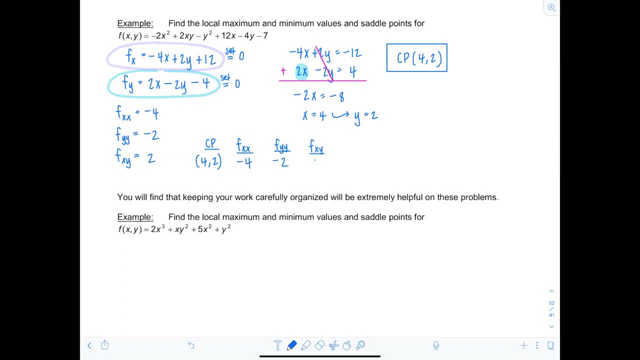 Then I want the second partial with respect to y, Then I want the second partial with respect to y, Then I want the mixed partial f sub xy. Then you figure out the sine of d. So you want to know if it's positive or negative. And when you organize the info this way, it's pretty easy, because when 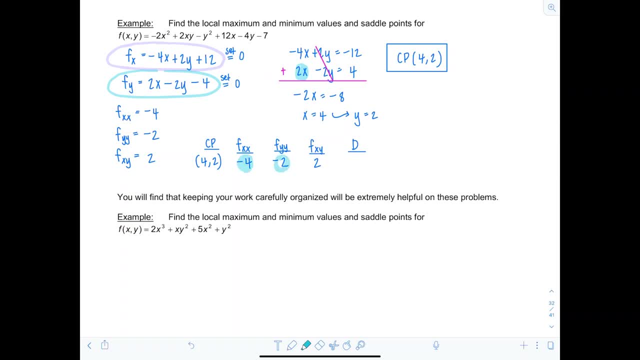 you find d. the formula is: you take this value, times that value and then you subtract that mixed partial squared So you can almost do it in your head. So that's going to be positive: 8 minus 2, squared, which is 4.. So this is positive: 8 minus 2, squared, which is 4.. So this is positive. 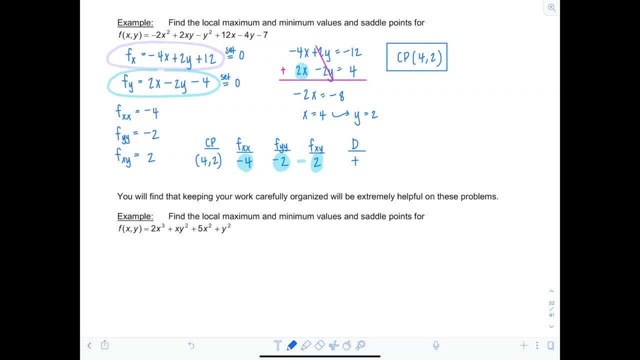 4, because x is positive. You don't really care what it comes out to be, You just want to know what the sine is, And then we're going to classify it. So notice here: since the value of d is positive and the second partial with respect to x is negative, then this is a relative max. 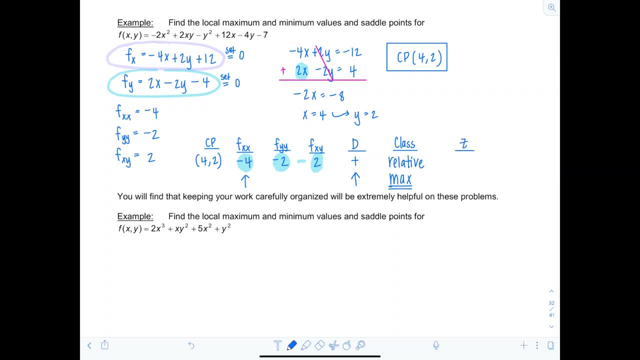 Okay, and then the last thing you do is you figure out what is that max value? So you're going to figure out what z is equal to, which is the same as evaluating f of X, Y. so f of 4, 2 is 13, all right, and then you could see if you had several. 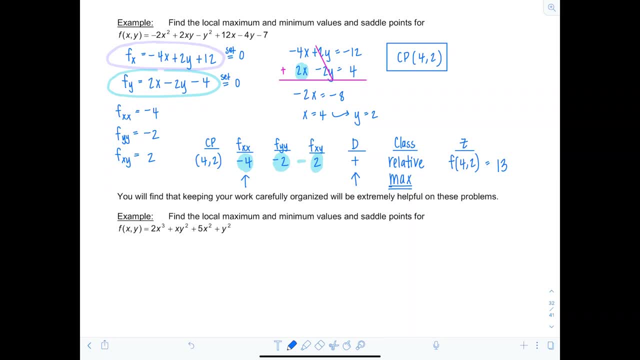 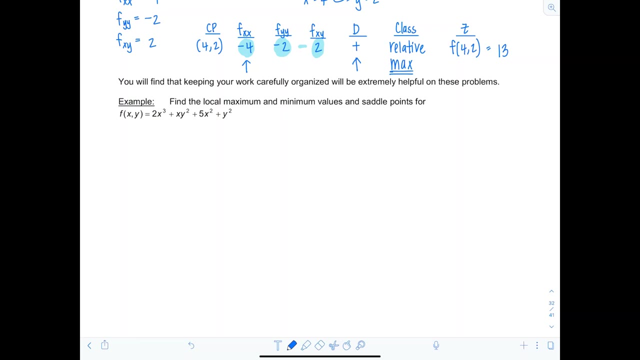 critical values, and you would just continue to list them below, and we'll do some examples right now like that. all right, let's look at another example this time where we have a little bit more going on and you have to keep your work organized, otherwise things will spiral out of control. so find the local maximum. 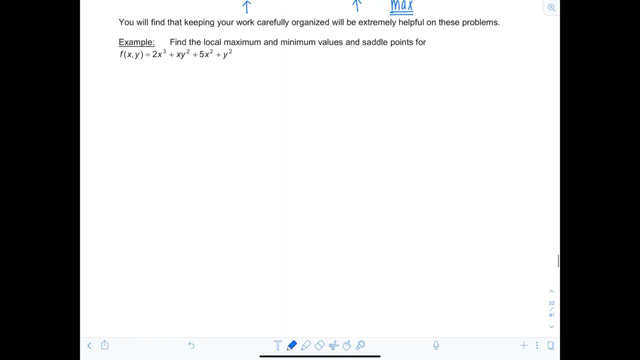 and minimum values and saddle points for the following function. so let's start off by getting our partial derivatives. so partial with respect to X, it's going to be 6x squared plus Y, squared plus 10x. and then partial with respect to Y is gonna be 2x Y plus 2y, and then let's go ahead and compute our second partials. 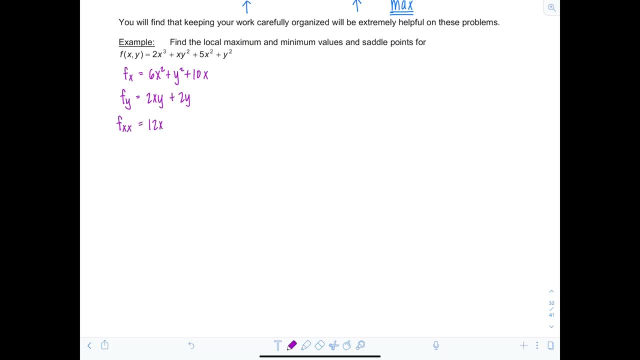 while we're at it. so f sub x- x is going to be 12, X plus 10, and f sub yy, 2x plus 2, and then our mixed partial f sub xy is 2y. Okay, very nice. Now remember we have to get our critical values first. 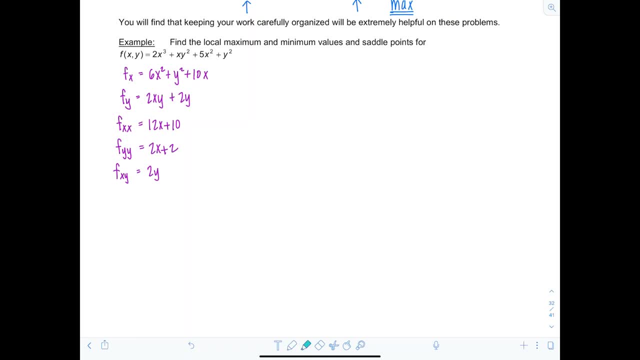 and this is a little more complicated, because look at this. partial with respect to x, So it's in terms of x and y, and I have quadratic terms, and then partial with respect to y doesn't look any better, if you ask me. I mean, we've got this 2xy going on, So which one is the less? 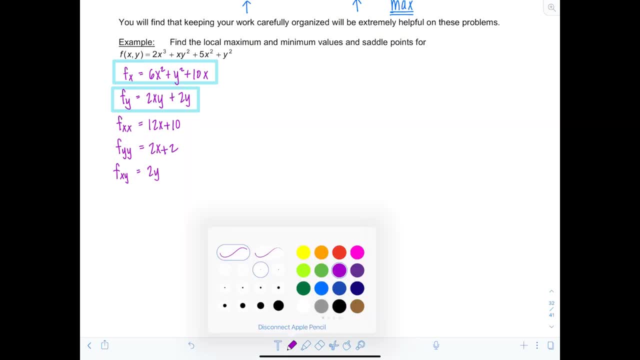 intimidating of the two, I would say partial with respect to y. So we're going to start off with that and remember they both have to simultaneously equal zero in order for us to have a critical value. So first I'm going to set f sub y equal to zero, which would mean that 2xy plus 2y is zero. 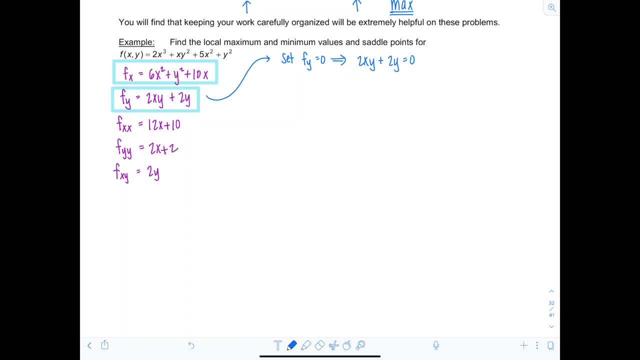 Okay, I can factor out a common factor. I can take a 2y out of both of these guys and then I have x plus 1 left over equals zero, And so now I can use the zero product property right, And I have two cases. So case one is going to be, if that first factor 2y. 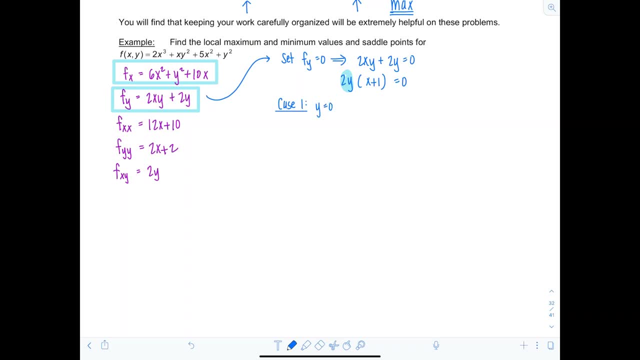 is equal to zero. Well, if 2y is zero, that means y is zero. Case two would be if that second factor equals zero, which would mean x plus 1 equals zero, And so that would be equivalent to x equaling negative. 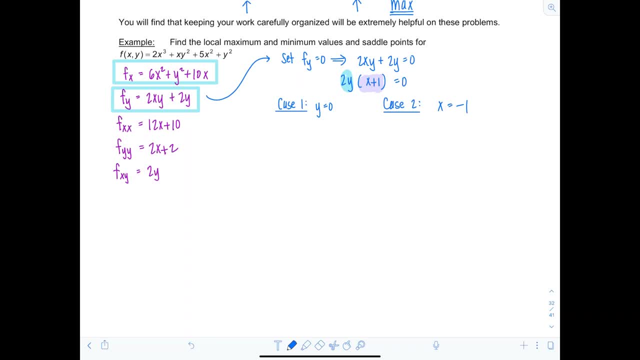 Now what I'm going to do is take each of these cases, substitute those values into the partial with respect to x and see what solutions I come up with. Okay, so for case one, if y is equal to zero, then substituting that into f sub x, partial with respect to x, I would get 6x squared plus zero. 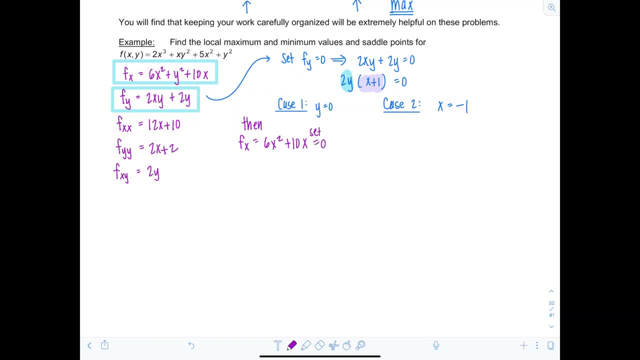 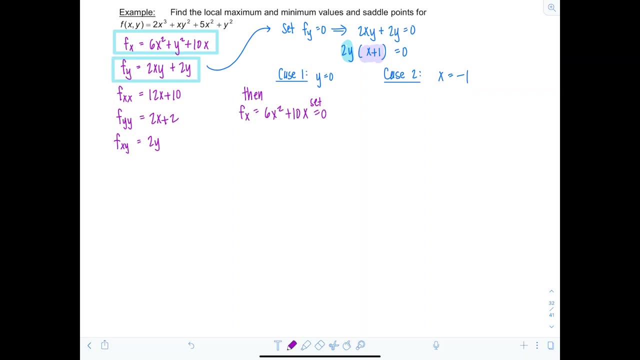 plus 10x is zero. I'm setting it equal to zero, right? Since I want to find a critical value, I want that to equal zero And I can just factor out the GCF, So I can take out a 2x and then I have 3x plus 5 is zero. 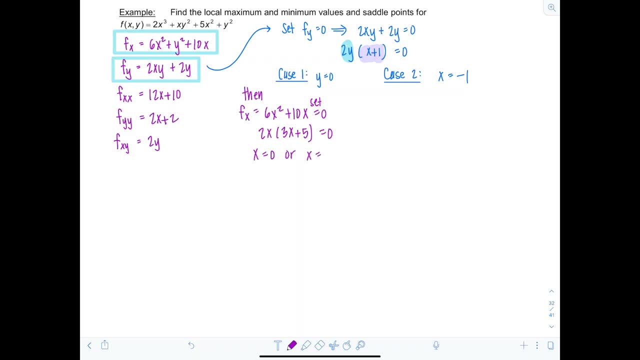 which means x is either equal to zero or x equals negative five-thirds, And remember we assumed y was zero for this case. So if x is zero, that means 0, 0 is a critical value And I have negative five-thirds- zero- as another possible critical. 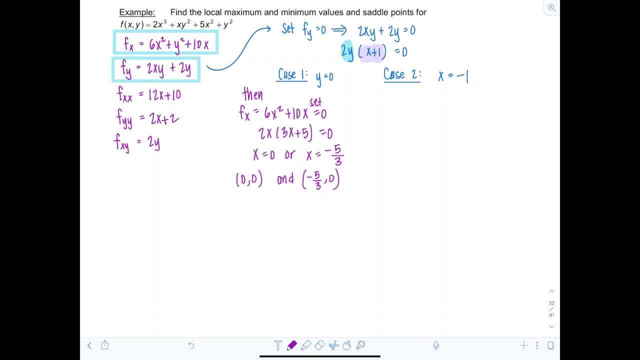 value. Okay, great. Now we're going to do the same thing This time, assuming x is equal to negative one, And again I have to go back to that partial with respect to x and substitute in negative one for x, and I'm going to set it to zero. 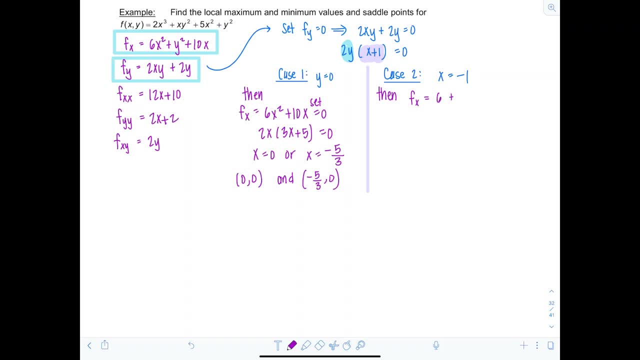 So if x is negative one, I'll still have six plus y squared minus 10.. And I'm going to set this equal to zero. That's y squared minus four equals zero, which means y is equal to 2 plus or minus 2.. And remember, in this case we assumed x was negative 1, so my critical values. 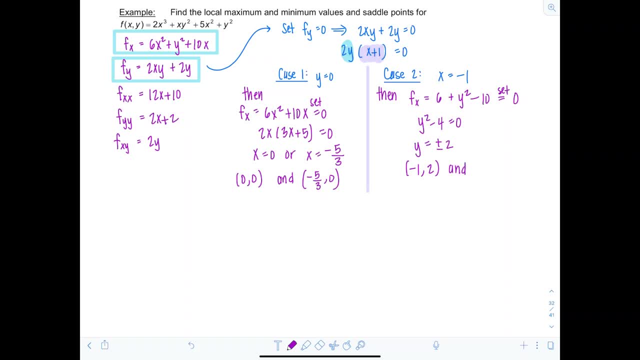 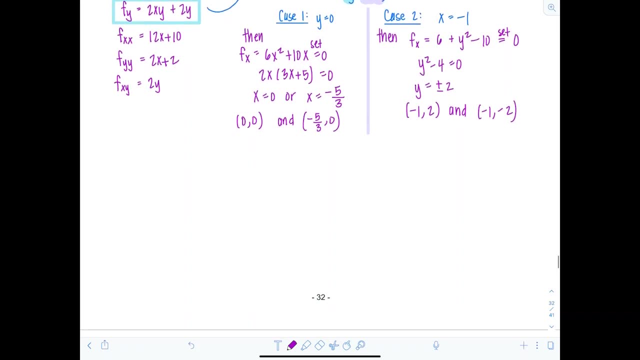 are negative 1, 2, and negative 1, negative 2.. So we've got four critical values to test this time, and you're going to see that this organizational method I outlined in the last problem is going to be very helpful. Okay, so here we go. So we're going. 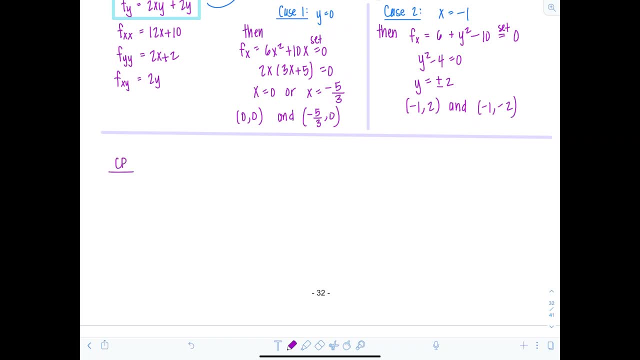 to list all of the critical points and then, second partial with respect to x, second partial with respect to y, your mixed partial f sub x, y, figure out if d is positive or negative, classify the critical point, and then you want to figure out what z is. 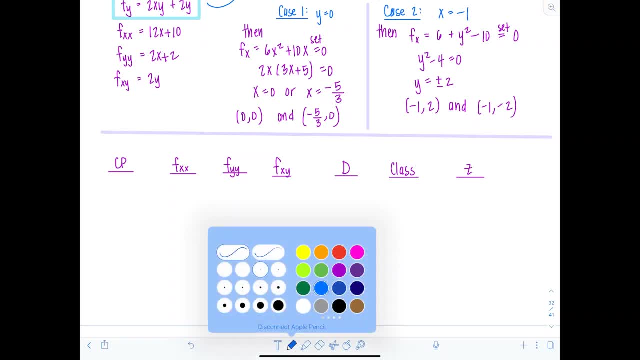 what the function value is. Okay. and then what I like to do is remind myself, right up above the column: so f sub x, x, that was 12x plus 10,. second partial, with respect to y, was 2x plus 2,. 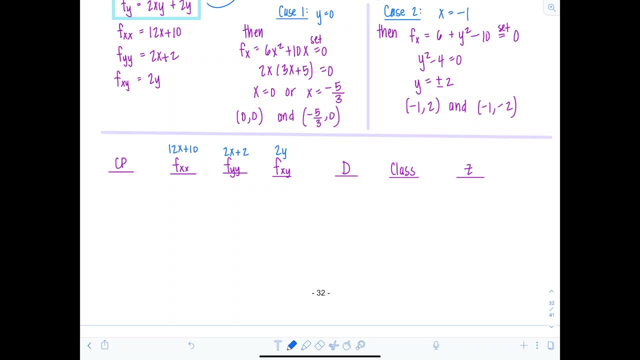 and then f sub x, y was 2y. Now let's go through. we'll list our critical values, our critical points. so we've got 0, 0, negative 5, third 0, negative 1, 2, and then negative 1,. 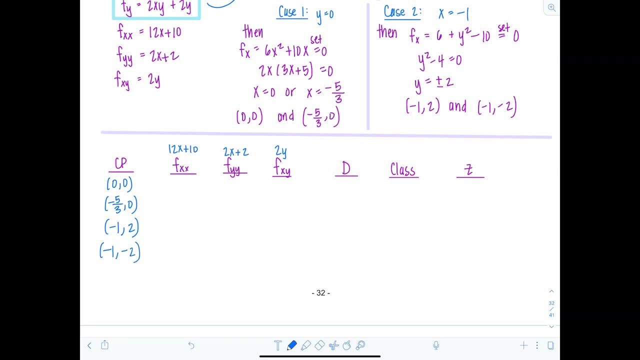 negative: 2.. All right, so let's see here. let's evaluate the second partial with respect to x. So if I plug in 0 for x, I'm just plugging in the x coordinate. right now This is going to be 10.. Let's just work our way. 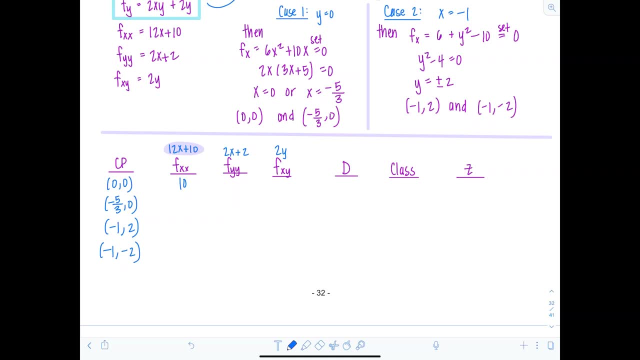 down the column. Next one's going to give me, if I plug in negative 5, third. so it's going to be negative 10 again. If I plug in negative 1, I'll have negative 2,, negative 2.. All right, let's fill in the next column now. So I'm going. 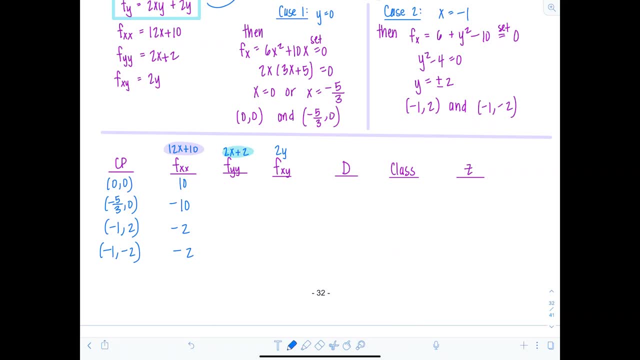 to substitute in the x coordinate for 2x plus 2.. So this will be 2, negative 4 thirds, and then these will both be 0.. Okay, moving on, now I'm going to substitute in the y coordinate. 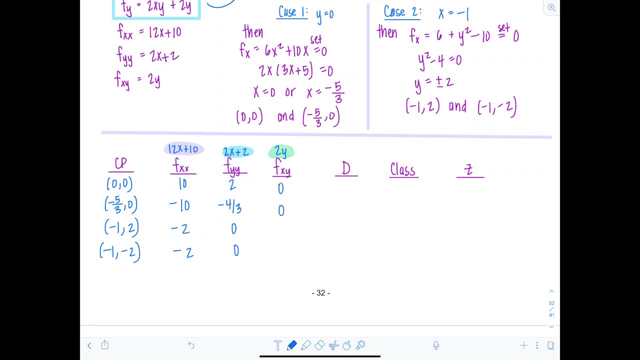 So this is going to give me 0, 0, 2 times y is going to be 4, 2 times negative. 3, 2 is negative, 4.. All right, now for d remember, you're going to multiply the values of the first. 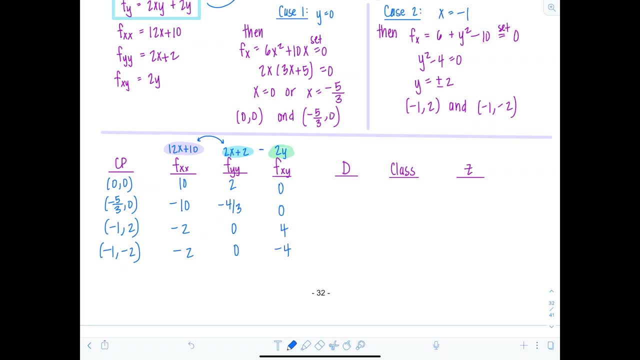 two columns and then subtract the square of this column. So 10 times 2, that's 20 minus 0, d is going to be positive, Negative. 10 times negative: 4 thirds, that's going to be positive minus 0 squared. that's still positive. Negative 2 times 0, that's 0, minus 4 squared. 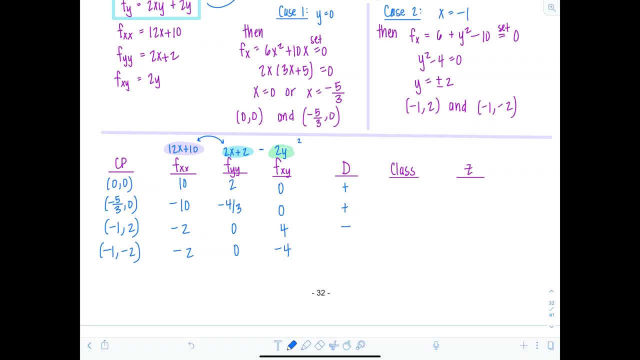 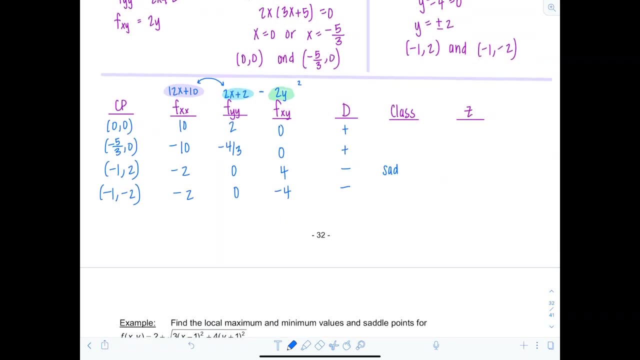 I'm subtracting Something from 0, it's negative, And then same thing for the last one. Okay, so anytime d is negative, automatically you know you have a saddle point. So these two are saddle points. Now, if d is positive, you have to check the value of the second partial with respect to x. So in 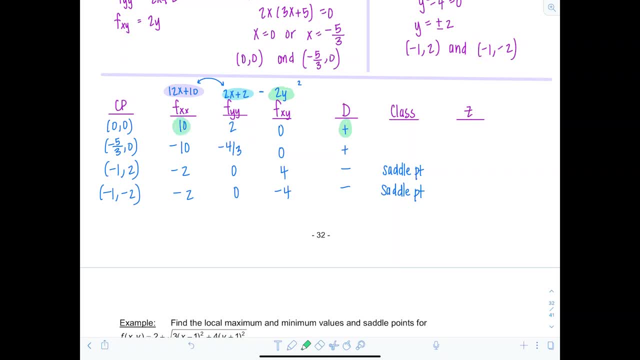 this case, d is positive and f sub xx was also positive, which means that 0, 0, you have a relative min. But then if you look at negative 5, third, 0, since the value of the second partial with respect to x. 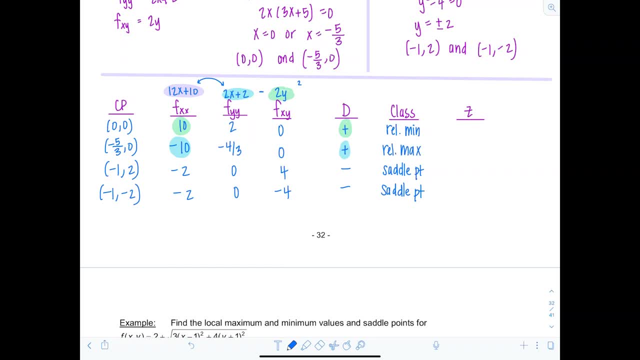 is negative. there we have a relative max. Okay, and then the last column. you want z or your function value f of xy. And just to jog your memory, f of xy is equal to 2x cubed plus xy. 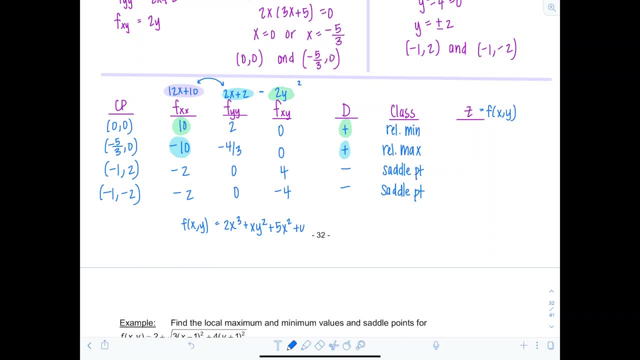 squared plus 5x squared. So you're going to substitute the value of the critical point. in that way, you can get what z or f of xy is equal to. And don't worry, I did it already for you And this is going to come out to: 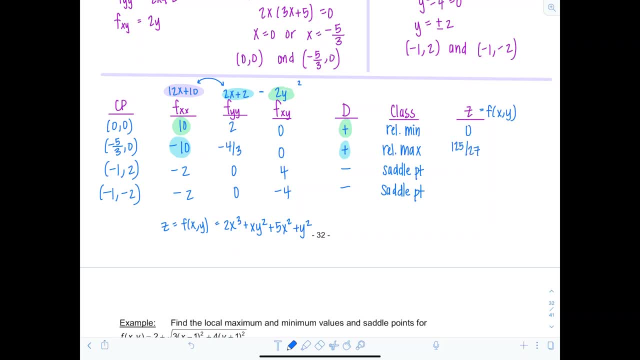 0,, 125 over 27,, 3, and 3.. Okay, very good. So now I think we have the process under control. I'm sure you're all still worried about the fact that I mentioned that sometimes the d test can be inconclusive or not apply, So now let's see what we would do in such a scenario. 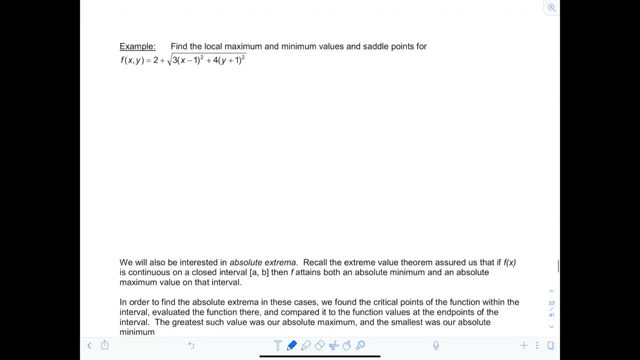 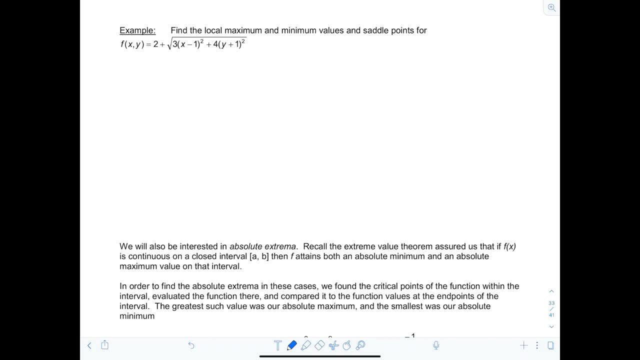 All right, so find the local maximum and minimum values and saddle points for the following function. So f of xy equals 2 plus the square root of 3 times x minus 1 squared, plus 4 times y plus 1 squared. All right, so let's go ahead and take our partial derivatives. 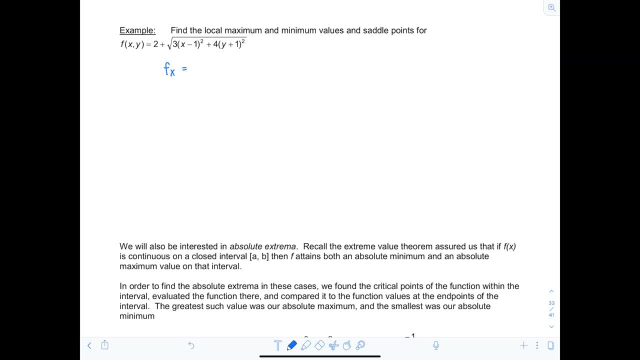 So partial derivative with respect to x. well, derivative of 2 is going to go to 0, and then I just have the derivative of this square root quantity. So remember our little shortcut: you just put 2 times whatever the radical is in the denominator, And then you 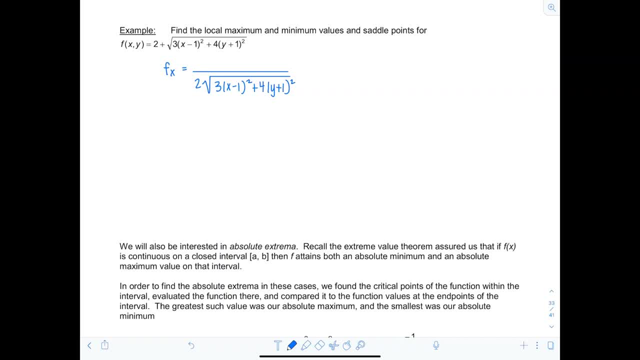 apply the chain rule and put the derivative of the radicand in the numerator. So derivative of everything underneath the square root with respect to x is going to be 6 times x minus 1.. And then this 2 and this 6 is going to cancel out and you just have a 3.. 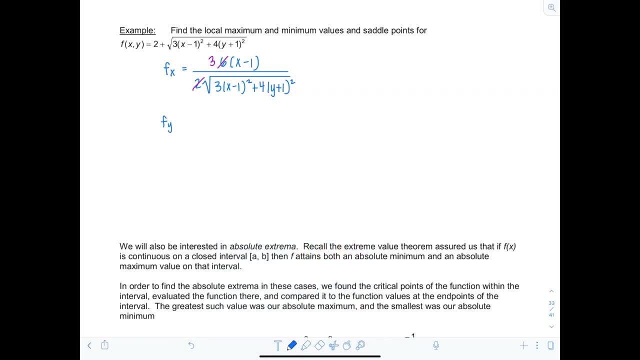 Okay, and then, similarly, not much would change right With that partial with respect to y. you would just have 8 times y plus 1, but then the 8 would cancel with the 2. So you have 4 times y plus 1 over radical, 3 times x minus 1 squared, plus 4 times y plus 1 squared. 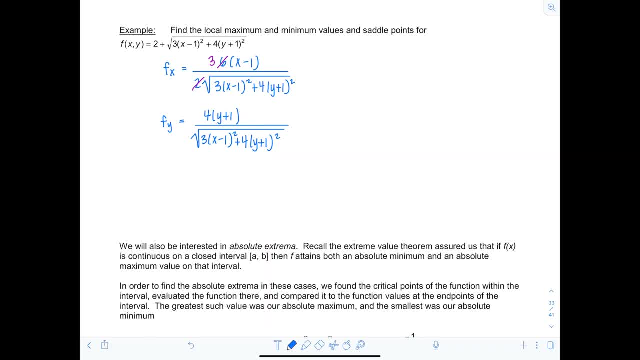 Okay, it looks lovely. Now what do we see here? Well, both of these are actually actually undefined at 1 negative 1.. That means also that they're never both going to be equal to 0. Because the only place where the partial with respect to x would equal 0 is if x is positive 1.. 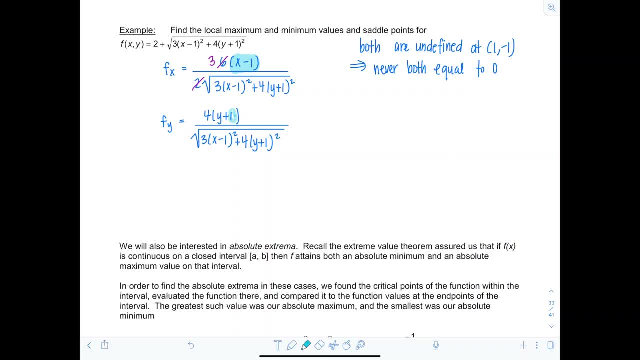 And if x is positive 1, in order for the partial with respect to y to also equal 0, then y would equal negative 1.. But that's exactly where they're both undefined at. Look at their denominators. Look carefully At 1 negative 1, they're both undefined. 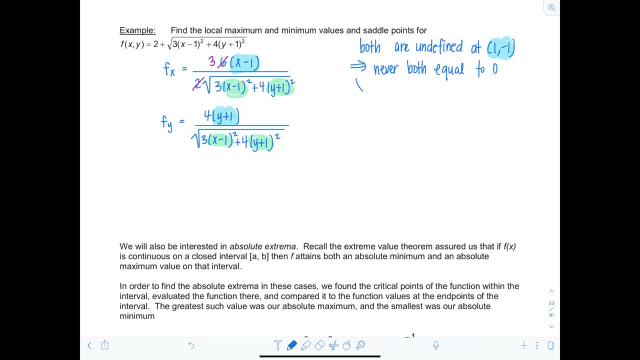 So what does this tell me? The D test does not apply. If you'll remember, we had to suppose, or we need the condition that the second partial derivatives are continuous On a disk and that these mixed partials have to simultaneously equal 0 at some point. a, b. 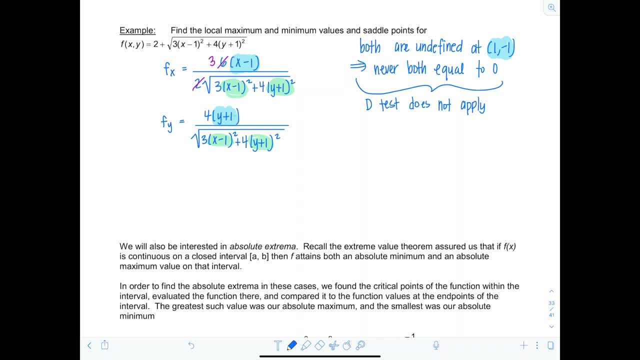 which is not possible here. Okay, well, is that point 1 negative 1 in the domain of the original function. Can I plug in 1 negative 1 into my original f of x y? Absolutely, Look, f of 1 negative 1 is 2 plus. this is going to be radical 3 times 0.. 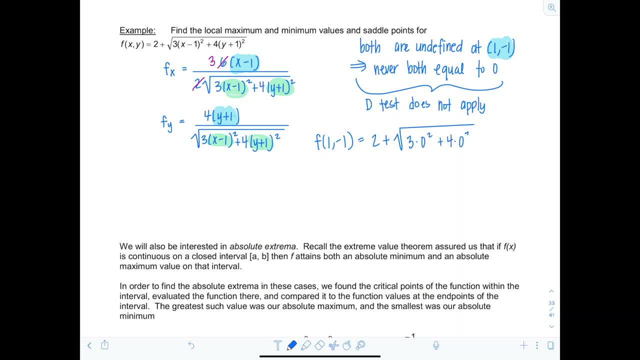 Plus 4 times 0, so this is just 2.. And notice: you have 2 plus the square root of some quantity, right? Well, when you take the square root of some quantity, it's never going to be negative. 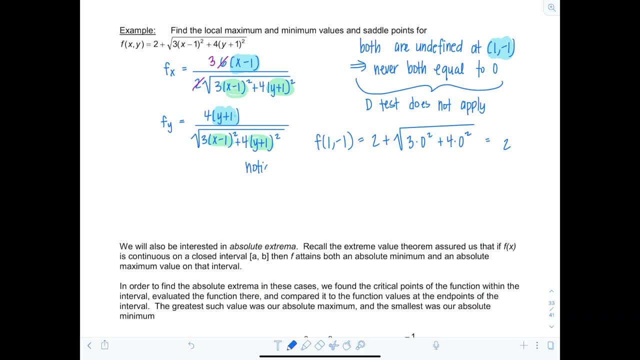 So notice that, interestingly, f is always greater than or equal to 2, right, So the local and absolute min value of 2 occurs at 1 negative 1. okay, and so in this case we were still able to figure out that F achieved a local or, even better, absolute. 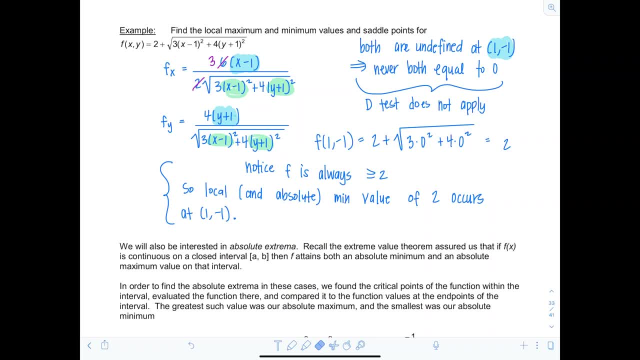 min at 1 negative 1 and that that value was 2 just by reasoning on the nature of the function. so when the D test doesn't apply, you'll be dealing with some kind of function that you can kind of gain information from just by observation and 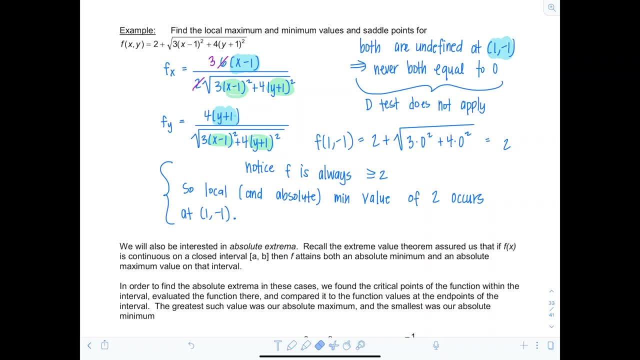 reasoning skills. okay, now I did throw out a word that we haven't used in a while when we did the last example, and that was an absolute min and, if you'll remember, our process for finding absolute extrema is a little bit different. so we use the extreme value theorem and remember that theorem. 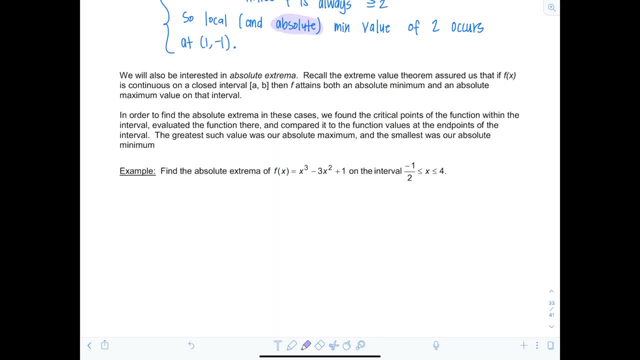 assures us that as long as our function is continuous on a closed interval from A to B, then for sure, for sure, we can find both an absolute min and an absolute max for the function on that interval. it's just that sometimes we also need to consider the endpoints in order for that to happen. so the process was as follows: 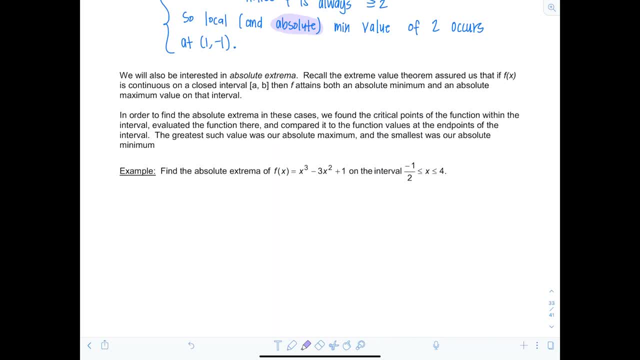 and we're going to actually revisit an example just to make sure we're all fresh and ready to go. you find the critical points. you make a table. you throw those endpoints of the interval in that table as well, evaluate your function values. largest is your absolute max, smallest is 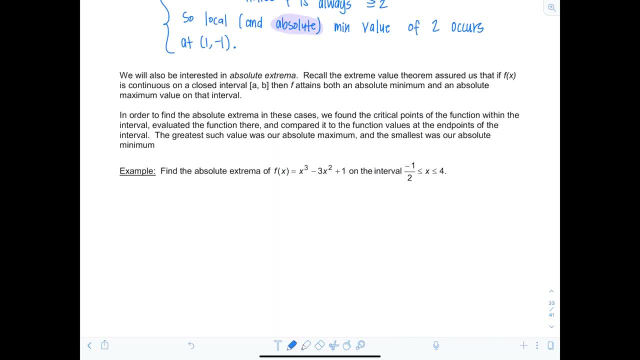 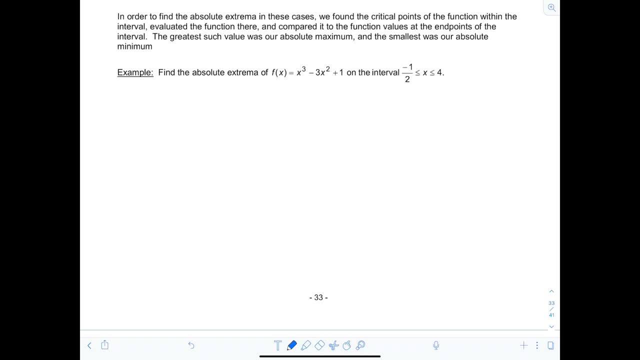 your absolute min. pretty straightforward. so here we go. find the absolute extrema of f of x equals x cubed minus 3x, squared plus 1 on the interval from negative one-half to four. so we've gotten a time machine. we're back in calculus 1. we're gonna start off by finding critical values. okay, so find a. 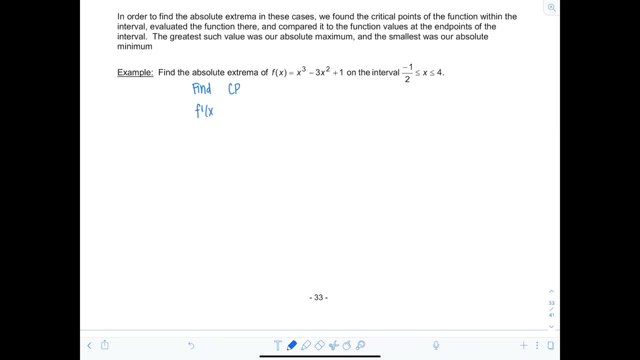 critical points first. So I need f prime of x. That's going to be 3x squared minus 6x. I'm going to set it equal to 0.. I can factor out a 3x and I have: x minus 2 is 0.. 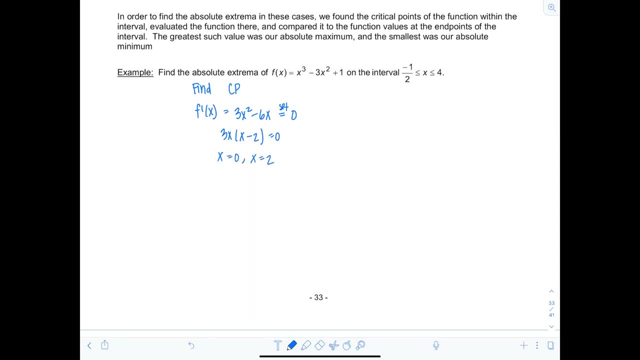 So I get: either x is 0 or x is 2.. Now, remember, there's another place I can get critical points for functions of a single variable, That's when f prime does not exist. But notice, f prime is a polynomial, so there aren't any. But always think about it. okay, It's dangerous if it doesn't even. 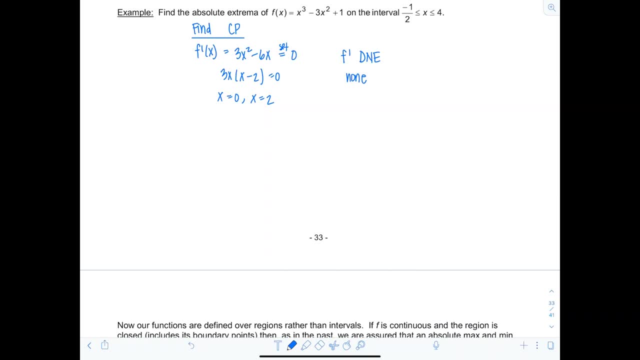 cross your mind. All right, when you're doing absolute extrema, you don't need to make a number line first, derivative test, none of that business. You just make a little table. So you have x, f of x. You put the critical values there: 0, 2.. Who else goes on the table? The 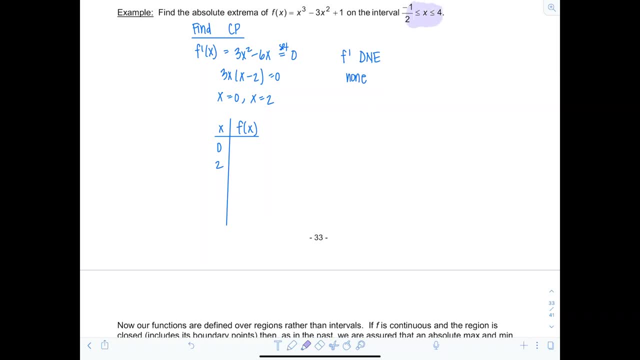 endpoints of your interval, because sometimes the absolute maximum it is achieved there, even if they're not critical values. So we'll throw in negative 1, half and 4.. All right, all of these values now get substituted into the original function. 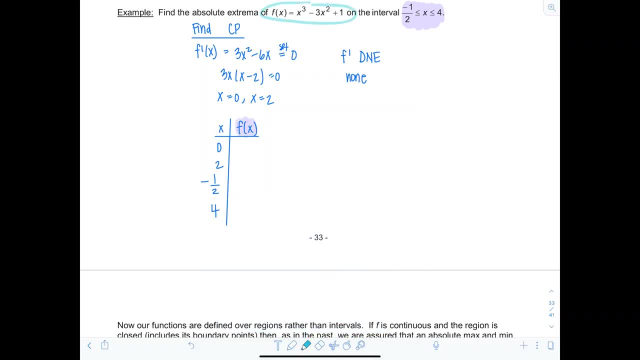 not the derivative You're plugging them into here- to f of x. okay, So 0 cubed minus 0 plus 1, that's 1.. 2 cubed minus 3 times 4 plus 1, that's negative 3.. And then the other two values come out. 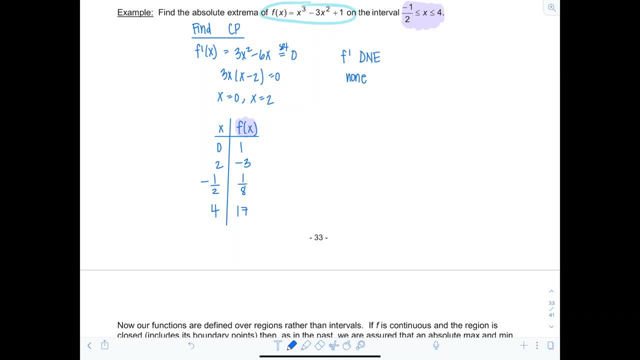 to be 1, eighth And 17.. And then now you just compare the values on the table. Well, it looks like negative, 3 was the smallest and 17 was the largest. So just summarize your findings here. So f of 2 equals. 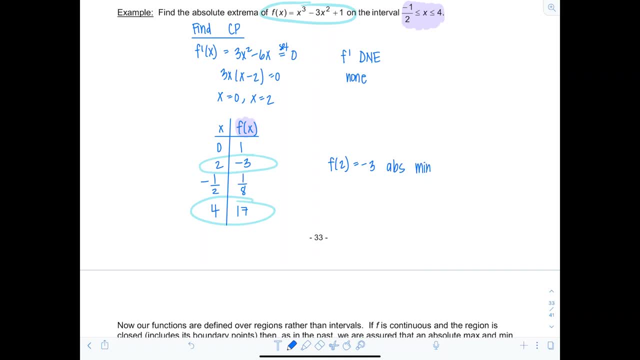 negative 3,, that's your absolute min, And f of 4,, which equals 17,, that's your absolute max. Okay, these are always pretty fun, So straightforward, right. Okay, now let's think about what happens when you have a function of. 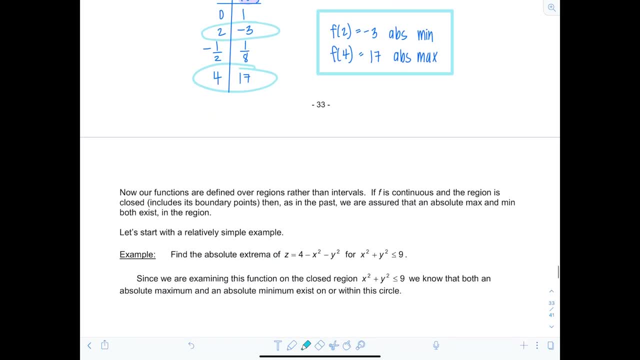 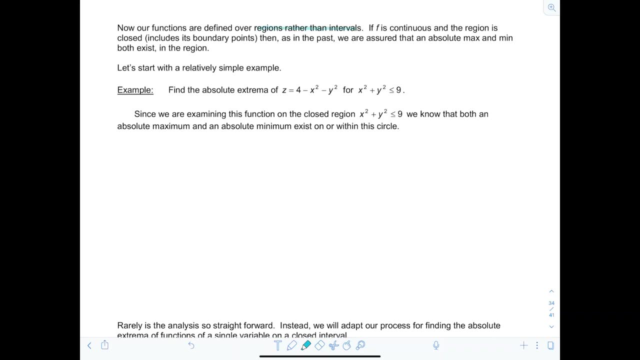 several variables because they're defined over regions rather than intervals, right? So if f is continuous and the region is closed, closed means it includes the boundary points, So that's equivalent to having a closed interval when you have a function of a single variable. 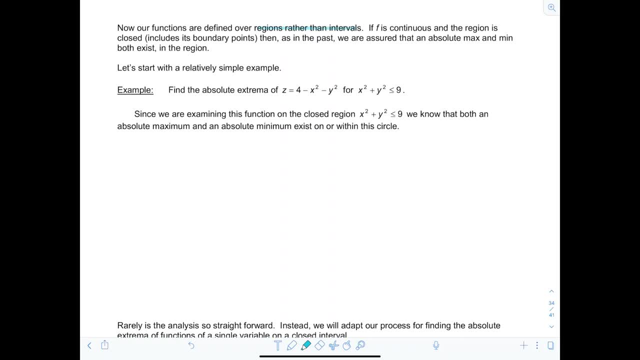 Then, just like in the past, we have a function of a single variable. and we have a function of a single variable, So we have the guarantee that there's an absolute max and min, that both exist within the region. So right now we're just going to look at a really simple example and then I'll show you the process. 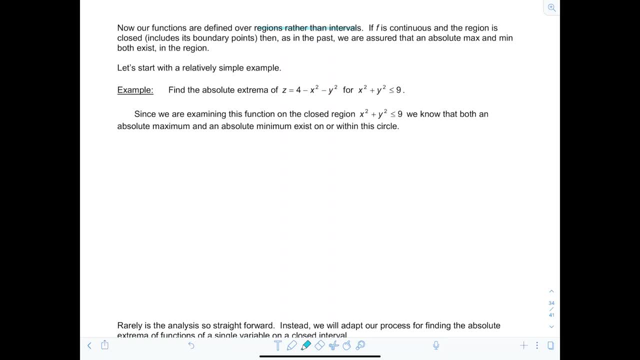 to apply for more complicated problems. okay, So find the absolute extrema of z equals 4 minus x squared minus y squared. for x squared plus y squared less than or equal to 9,. okay, So I'm only examining this function On the closed region. x squared plus y squared is less than or equal to 9.. So I know that I will. 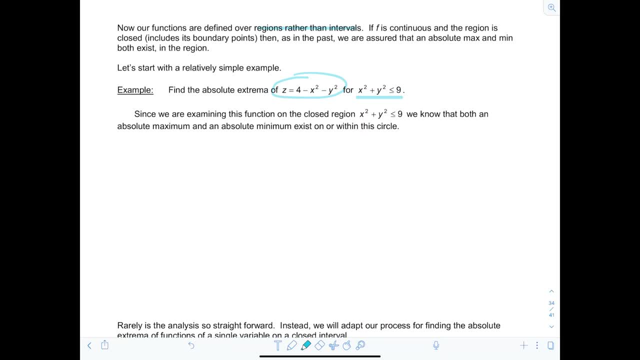 definitely find both an absolute max and an absolute min on or within that circle right, x squared plus y squared, less than or equal to 9, that's a circle. Radius is 3, centered at the origin. Do you know what the graph of z equals? 4 minus x squared minus y squared is? It's a. 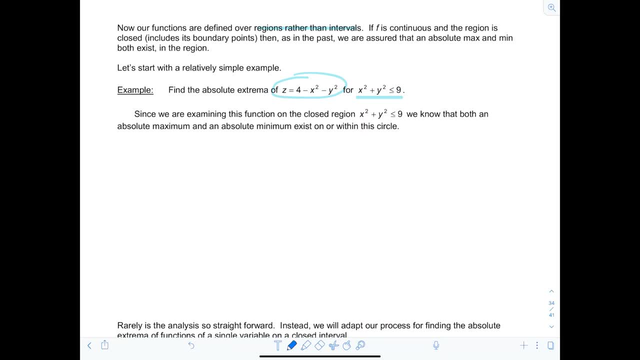 paraboloid right Opening downward, and it's been shifted up four units. Now all that graphing is going to come into play, So let's graph it. And it's also helpful because I know up here 1, 2, 3, 4, right, 1, 2, 3, 1, 2, 3, okay. 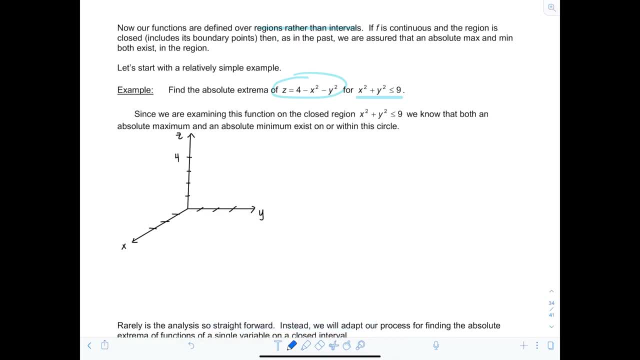 Okay, It's also helpful to know here for the paraboloid, when it hits the x-axis, it's going to be a paraboloid, So it's going to be a paraboloid x- y plane. that's going to be when z is equal to 0, right, So you would have 0 equals 4. 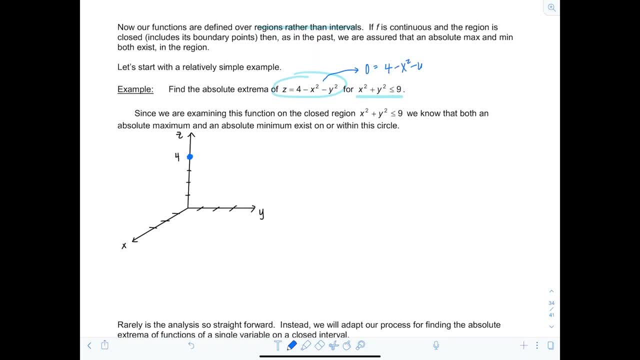 minus x squared, minus y squared. So when z is equal to 0,, the intersection is going to be a circle of radius 2.. So there's the paraboloid. Let's make sure it looks beautiful. Oh, yes, Okay. So I want to know what is its absolute max? 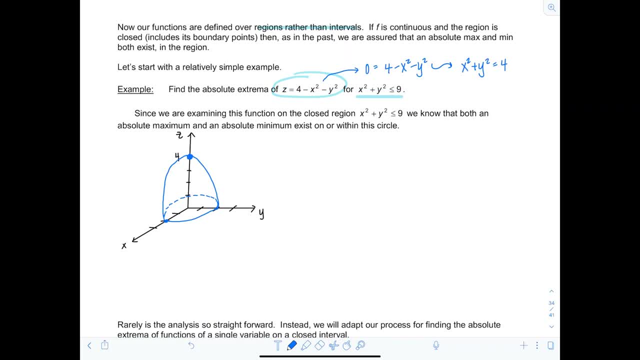 and absolute min, if I'm only considering values for x and y that get substituted in on a circle of radius 3.. Okay, Because I know. what do I know about the paraboloid? Well, I know it's going to keep going. 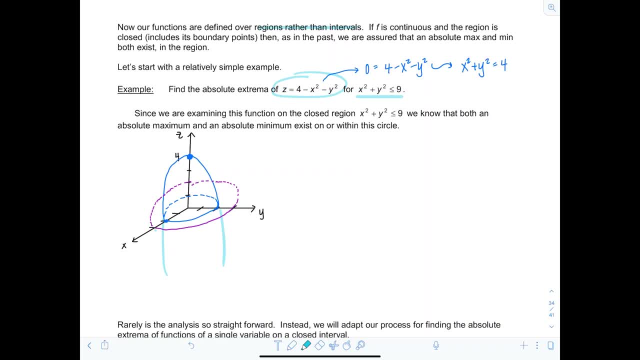 down forever, right? So really there's no absolute min. But if I restrict myself to only looking at values for x and y that satisfy that x squared plus y squared is less than or equal to 9, then I'll be able to find it Okay. Just looking at the graph can you already tell. 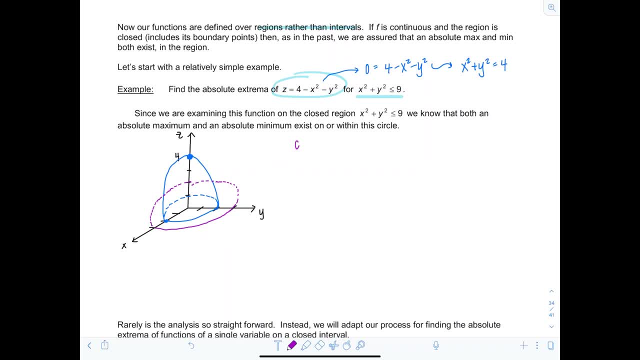 where the absolute max is going to be. The absolute max occurs at 0,0, and we can see that f of 0,0 is equal to 4.. Right here, 0,0 equals 4.. That's pretty straightforward. Now let's see if we could figure out any critical points. You could have found this: 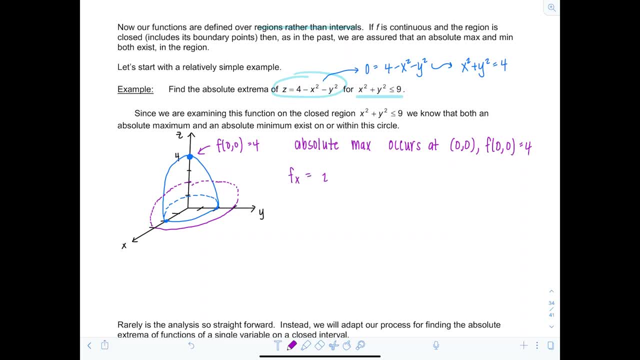 another way. So if you take the partial with respect to x, you get negative 2x. Partial with respect to y is also negative 2y. if you set both of these equal to 0, you would get that x squared is 0, y is 0, which means that 0, 0 is a critical point, But that's our only critical point. So how? 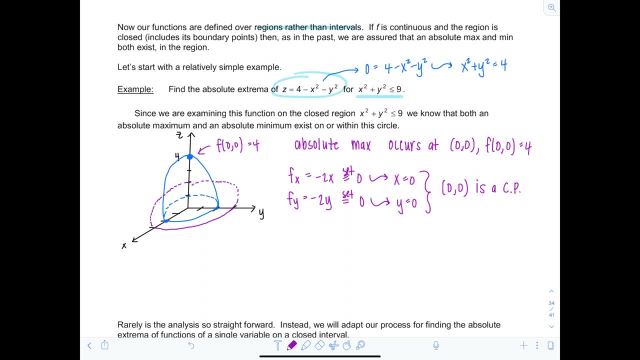 am I going to find the absolute min? Well, just look at your graph. okay, Your absolute min is going to occur when you're at the very extreme edge of this circle. x squared plus y squared equals 9.. Because z is equal to 0 when x squared plus y squared is equal to 4.. But notice this: 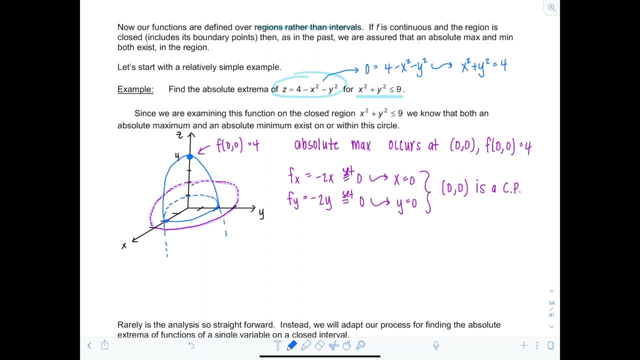 paraboloid, it's going to keep going down, down, down, down, down, down down. And you could plug in a value here into z. So the absolute min is 0.. occurs at all of the points on the boundary of the circle. on x squared plus y squared equals 9.. 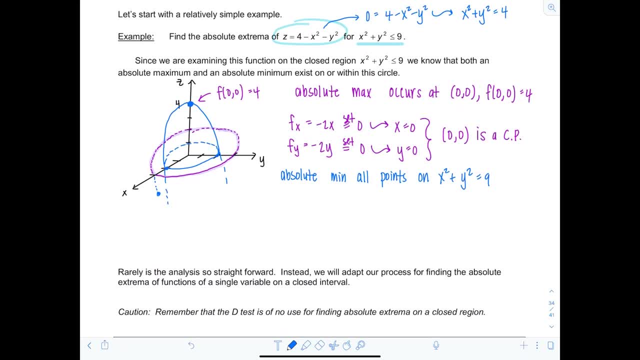 And you could see, I could play around with my function a little bit and find it quite easily, because z equals 4 minus. let me factor out that negative x squared plus y squared, And so, since the absolute min occurs when x squared plus y squared is 9, I'm just going to 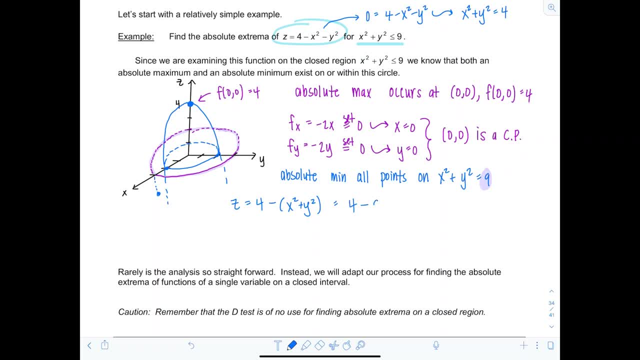 substitute that in, So that's going to be 4 minus 9, which is negative 5.. So that's our absolute min, and there's infinitely many points where it's going to occur. All right, let's graph it so we. 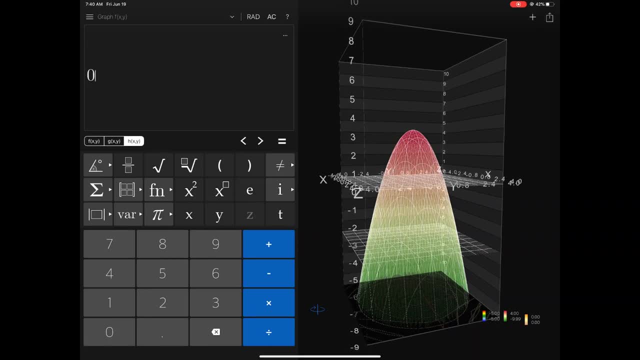 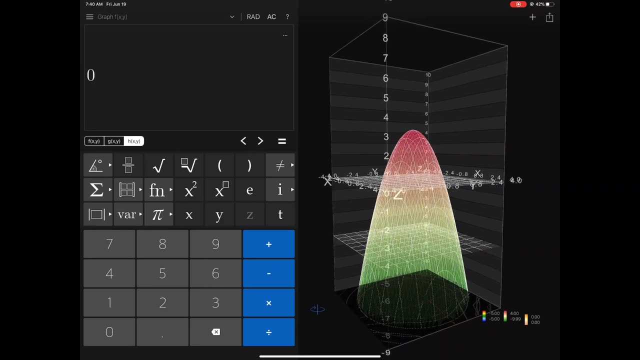 get a better perspective, All right. so, if you'll notice, here we have the graph of that paraboloid. z equals 4 minus x squared, minus y squared. And then I've added in two planes, one where z is equal to 0, and the other one where it's equal to 0. And so I've added in two planes. 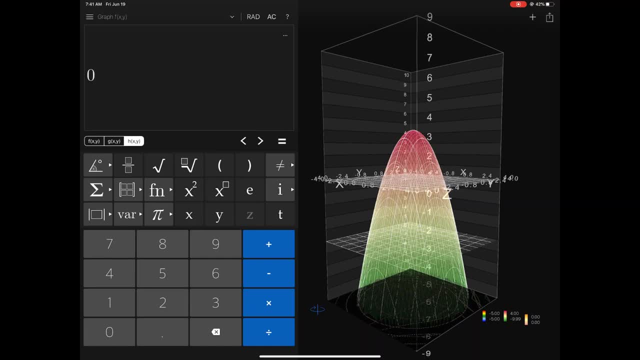 one where z is equal to 0, and the other one where it's equal to 0. And so I've added in two planes: zero. so that's the xy-plane, and then below is where z is equal to negative five. So if you'll, 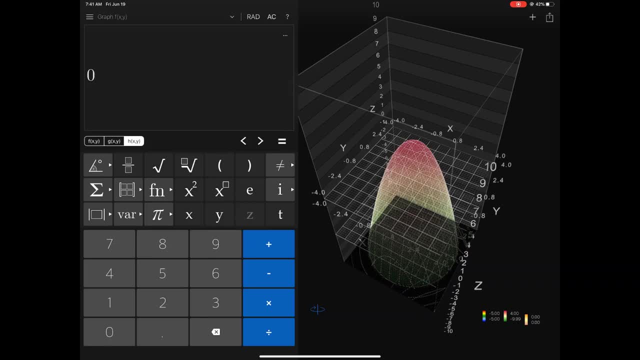 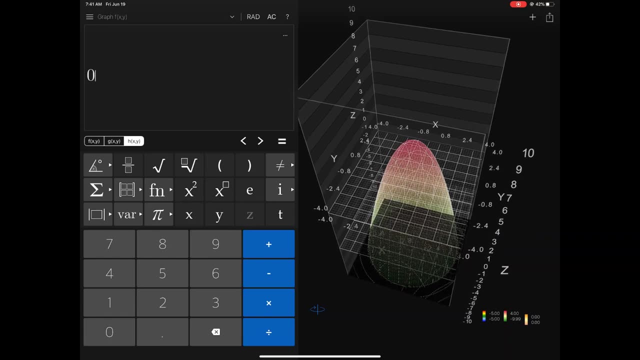 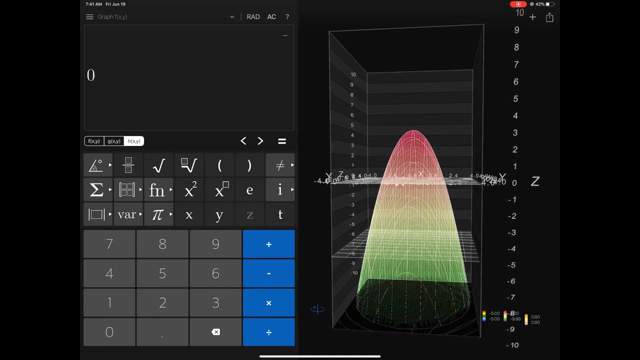 notice, here, at this plane, up above the xy-plane, the paraboloid intersects it at the circle. x squared plus y squared equals four. But then notice, if we're allowing x squared plus y squared to be as large as nine, now I can go below the z-axis, below the xy-plane, and that's where we 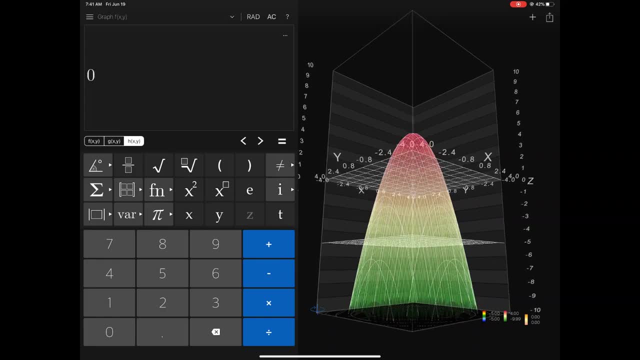 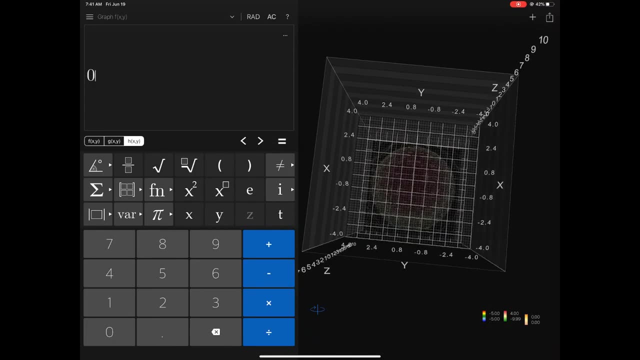 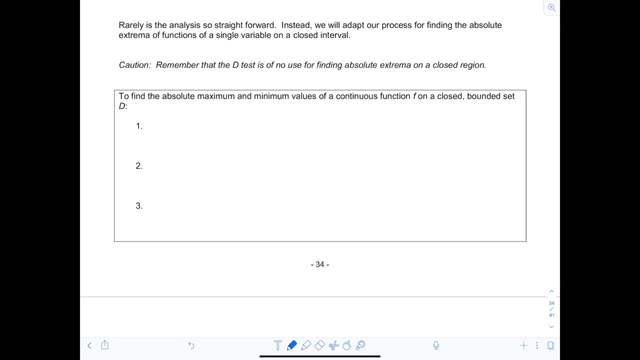 achieve that value that I've shown here, where z is equal to negative five And it intersects the paraboloid at a circle of radius three. So if you look down this way, you can see that. All right, Okay, hopefully that was helpful. When finding absolute extrema, it's very rare for our analysis. 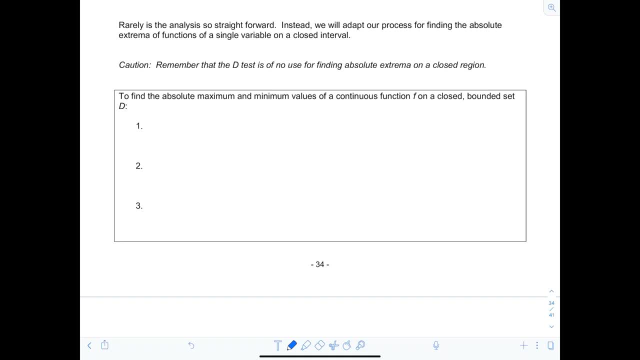 to be as straightforward as it was in the previous example. So I'm going to give you a process now for how to find absolute extrema for functions of several variables, And it's going to be pretty similar to how we did it for functions of a single variable. 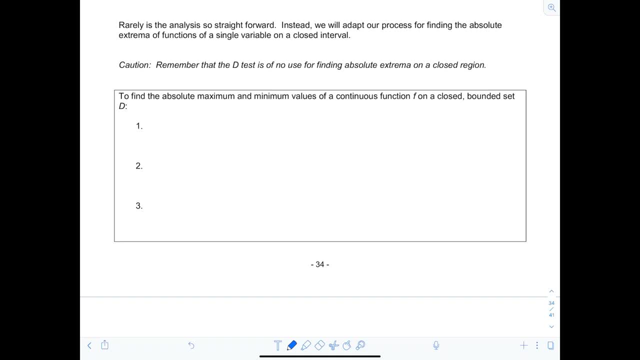 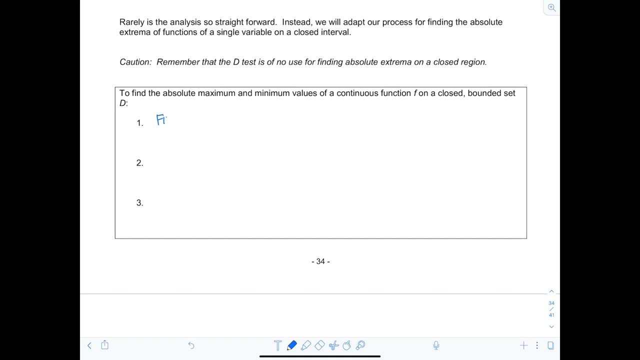 Now remember: the D-test is not useful when you're finding absolute extrema on a closed region. The D-test is only used for local extrema. Got it Okay? so here's the process. To start off, you have to find the critical points inside the region. So same beginning as before. 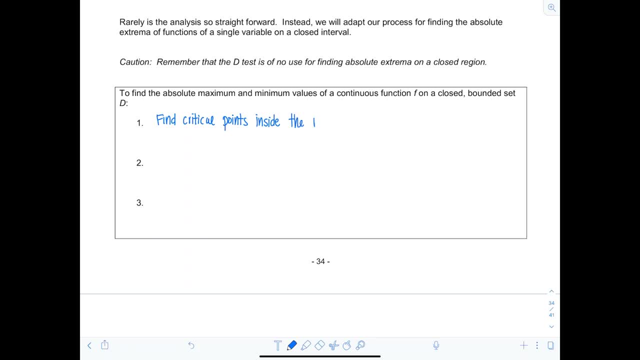 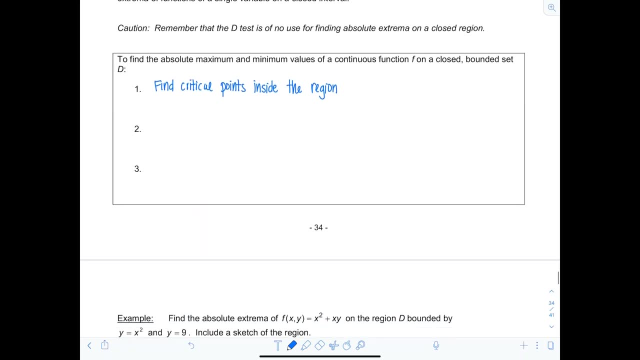 So you take your partial solve where they're both equal to zero or don't exist. From there you have to find the points where extreme values may occur on the boundary. That's equivalent to checking the endpoint. So you have to find the points on an interval And you have to make sure you include corner points. 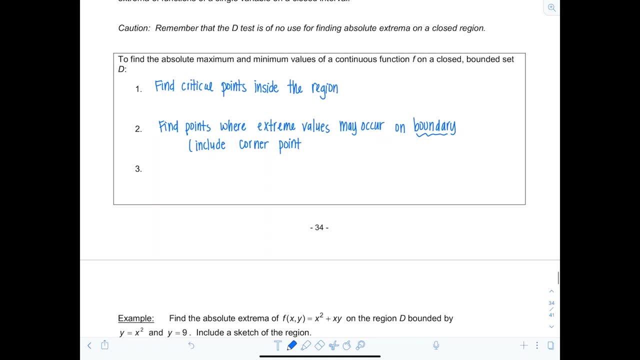 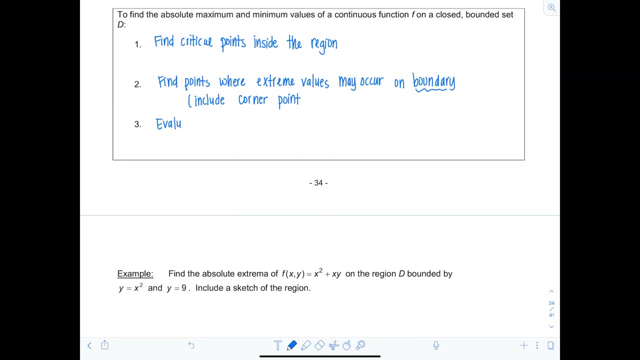 I'll show you what I mean by that in a minute. And then, just like for a function of single variables, you would evaluate your original function, Evaluate f of x, y at all these points. So you can make a little table, organize your info. 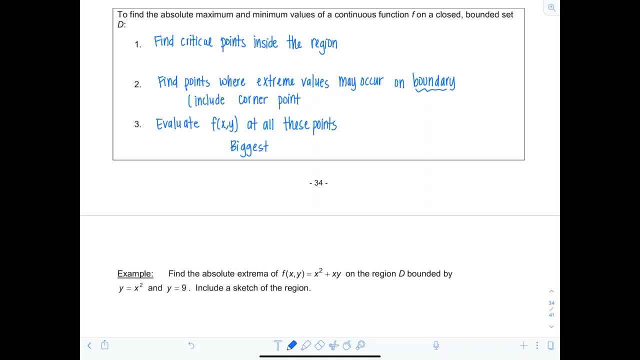 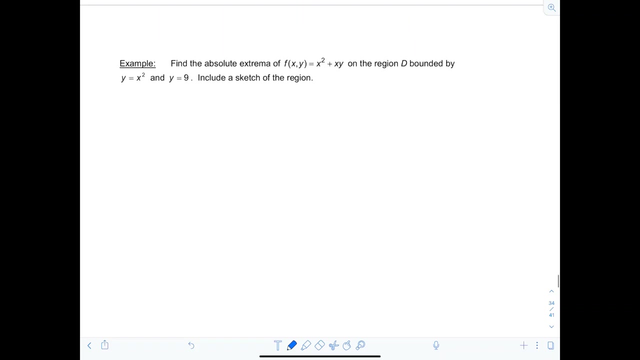 And guess what? The biggest value, that's your absolute max, and the smallest, that is your absolute min. All right, so let's look at an example. Find the absolute extrema of f of x, y equals x squared plus x- y on the region D that's bounded by y equals x squared and y equals nine. 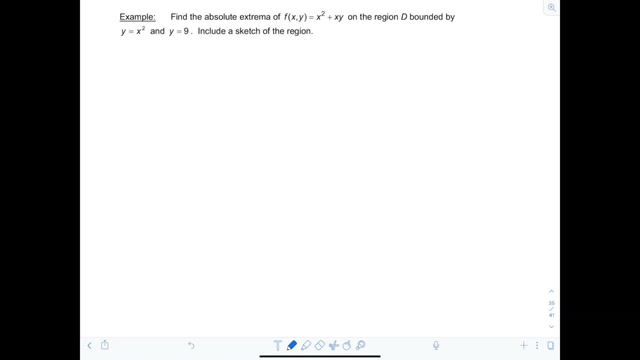 Include a sketch of the region. I mean, even if they didn't tell you to include a sketch, you need to do it, okay, Otherwise you won't be able to find the boundary. So y equals x squared and y equals nine. Hopefully that's easy for you to sketch. 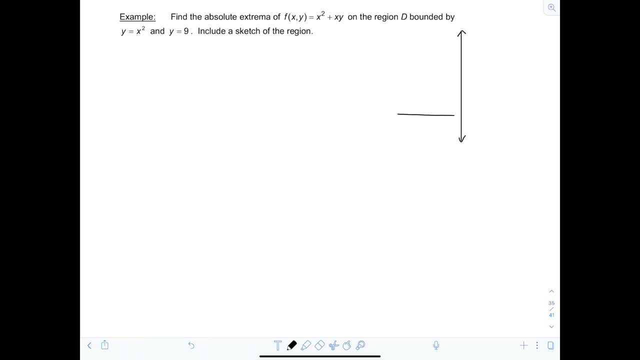 We've got a parabola that's opening upward Center, or its vertex, excuse me, is at the origin And y equals nine. That means they're going to intersect when x is 3 and negative 3, right 1, 2, 3, 1.. 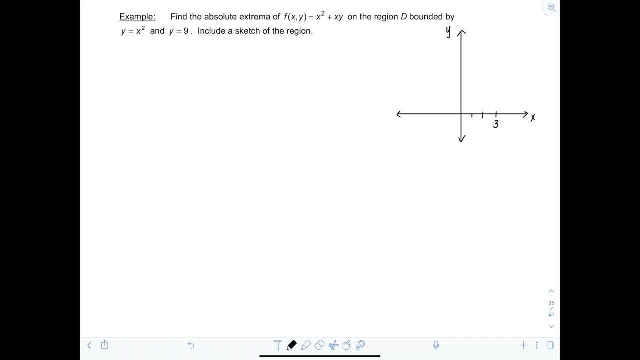 1, 2, negative 3.. And we'll say this is nine. okay, So I have y equals nine. That's part of my boundary, Okay. good, We'll just move this. There's nine. Okay, that's y equals nine. 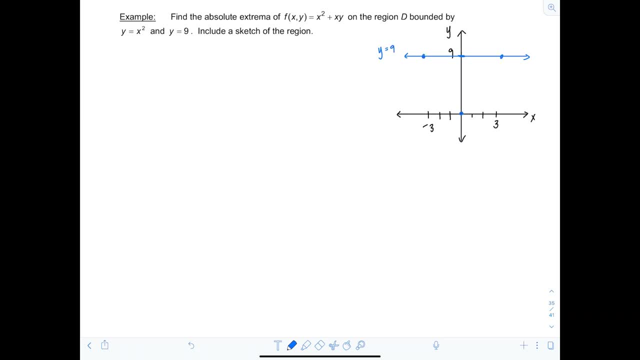 And then the parabola is going to intersect there as well. So we want to find the max value of the function Only looking at values inside here, inside this region. So you could imagine, like f of x, y lives above and below this region. 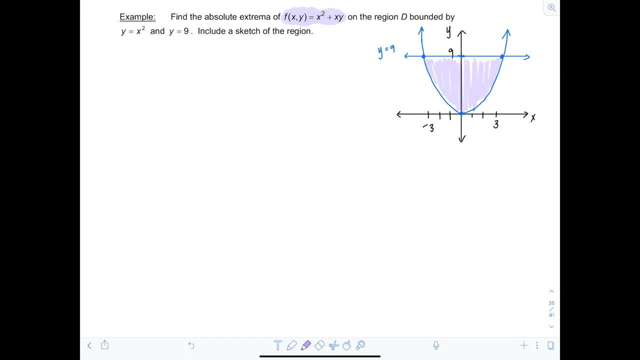 And I want to figure out when z is a max, when z is a min, Only looking at values above or below this region. This is the region D. Okay, so let's start off. We're going to find our critical points. 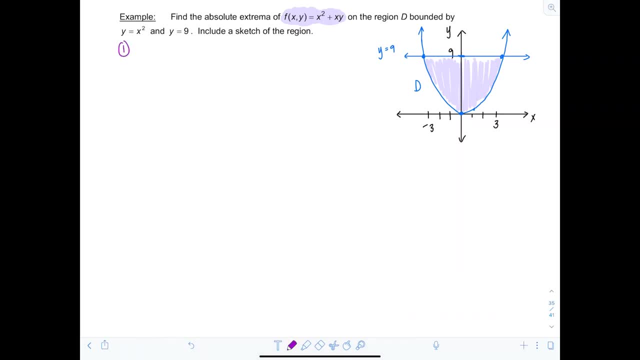 That's familiar. So we're going to look at our partial derivatives with respect to x and y. So partial with respect to x, that's going to be 2x plus y. Partial with respect to y is equal to x. I'm going to set both of these equal to 0.. 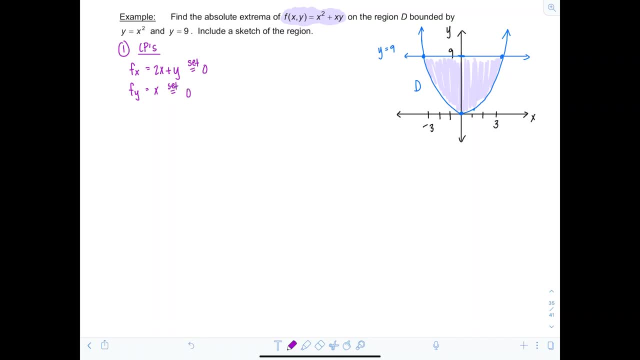 Well, second equation: easily I can see x is going to be 0. And then if x is 0, that means y has to be 0 from the first equation. So 0, 0 is a critical point. Okay, now I need to find potential critical points on the boundaries. 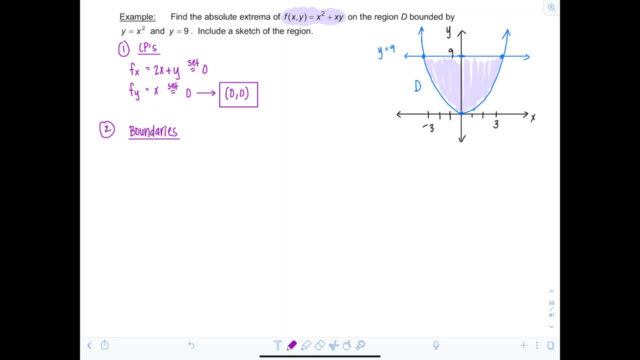 Well, how many boundaries do I have? How many different equations do I have that bound the region? Well, I see two. One is the parabola: y equals x squared And the other is the line y equals 9.. 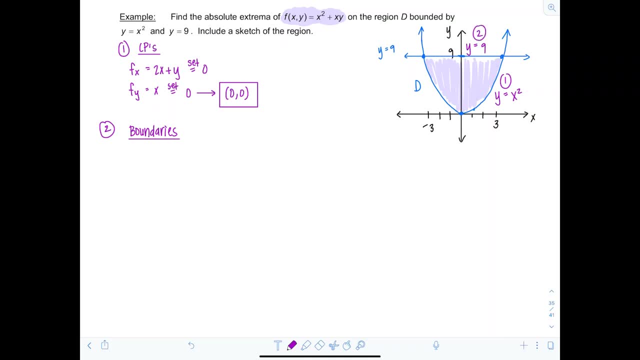 Those bound the region D. So we're going to have to test on each of them. How do you do it? Well, first, let's say we're going to test on: y is equal to x, squared. Okay, now I come back to my function, f of x- y, and I'm going to evaluate f of x- x squared. 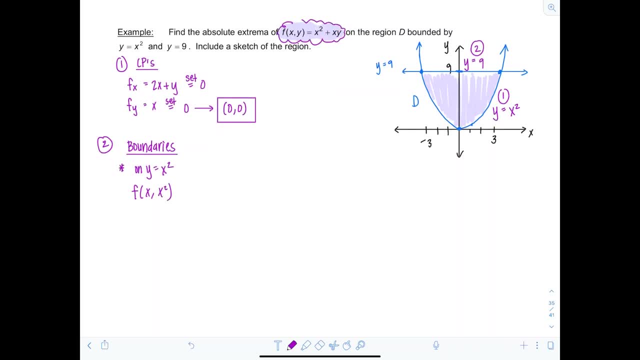 So go back here to the original and I'm going to substitute x squared in for y, because I'm testing on that boundary, So I'm going to have to do that. So I'm going to have x squared plus x cubed. 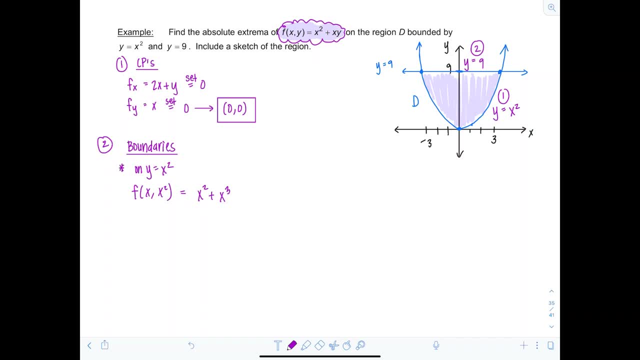 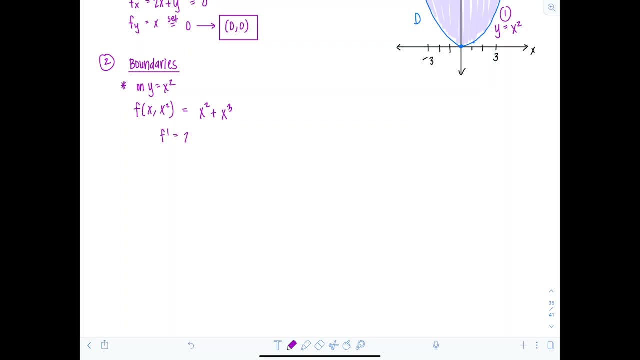 And then now pretend you're back in calculus 1, and you want the critical points of this new function here. So okay, we're going to take the derivative. So f prime is going to equal 2x plus 3x squared. 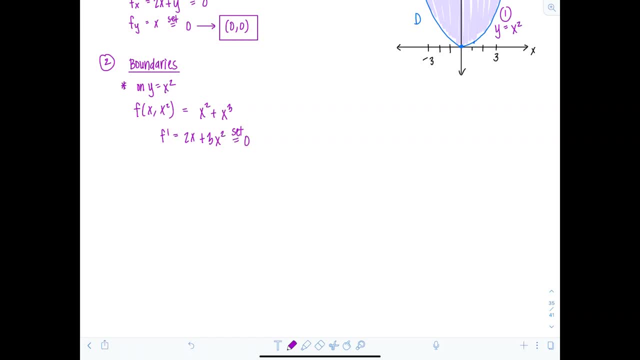 I'm going to set this equal to 0.. Take out the GCF. What can I take out Just an x, And then I have 2 plus 3x equals 0. So x is 0. Or x is negative 2 thirds. 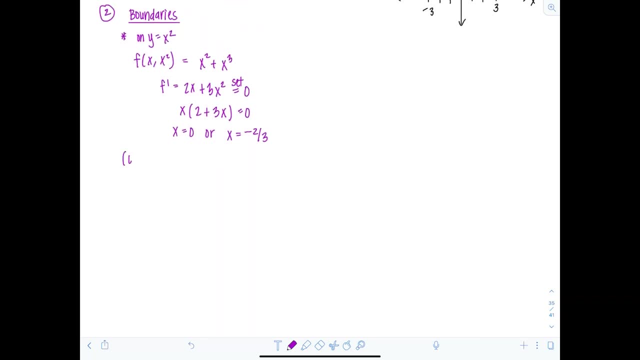 All right. So for the critical points, I have 0.. And then, remember, we tested on the boundary: y equals x squared. So to get the y coordinate, just square the x coordinate, Or I have negative 2 thirds. And since y is x squared, y would be 4 ninths. 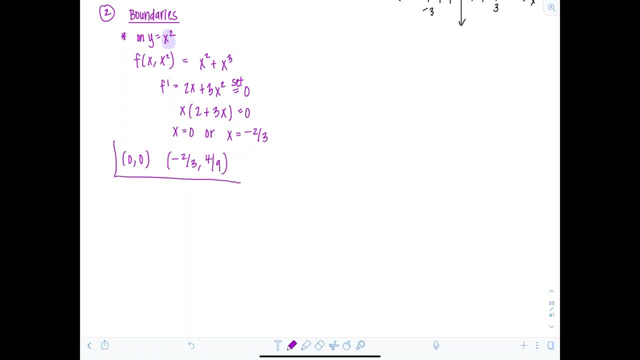 All right, So here's two more. Actually, we already knew about 0, 0,, didn't we? That's no new news, It's for us, Okay. So that boundary is taken care of. Now I have to check on the other boundary, which was y equals 9.. 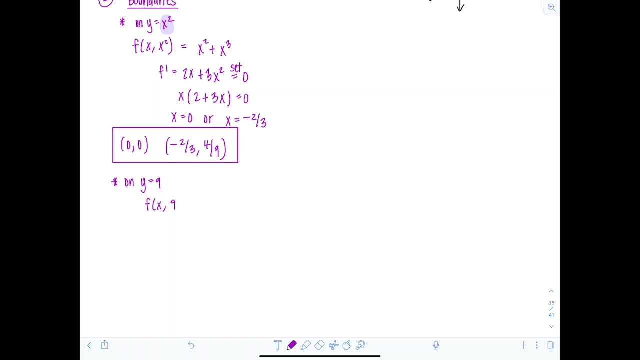 So I'm going to have f of x, comma 9.. And then, substituting that back into f of x- y, I'm going to end up with x squared plus 9x. Take the derivative. We want critical points, So we'll have 2x plus 9.. 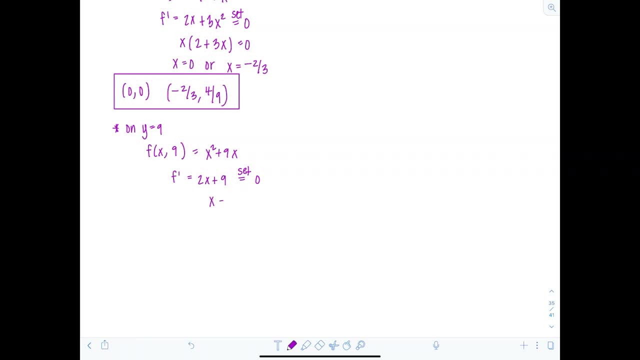 And then I'm going to set this equal to 0. So I get: x is equal to Negative 9 halves, And if x is negative 9 halves, y is 9.. But look at this: x is negative 9 halves. 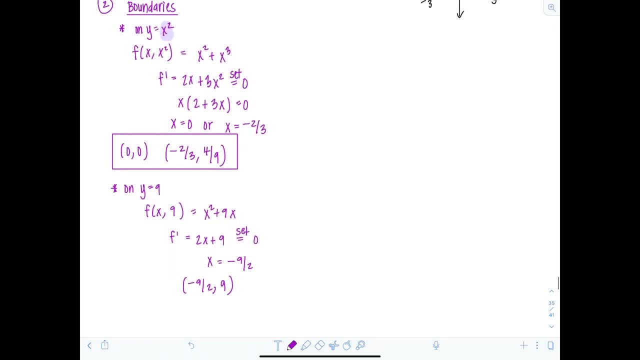 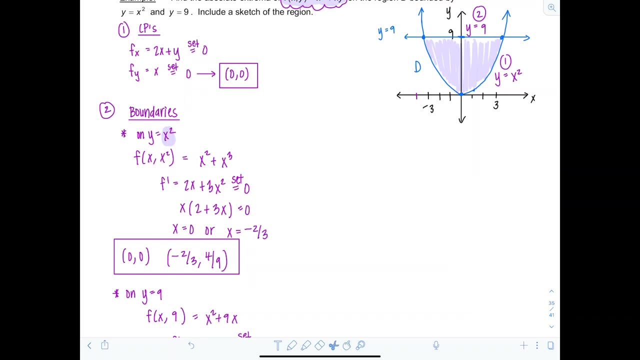 That's negative 4.5, right, We'll look at our region D. This is why you always need to graph it. Negative 9 halves is going to be outside of the region. So this is a no-go Discard, this value. 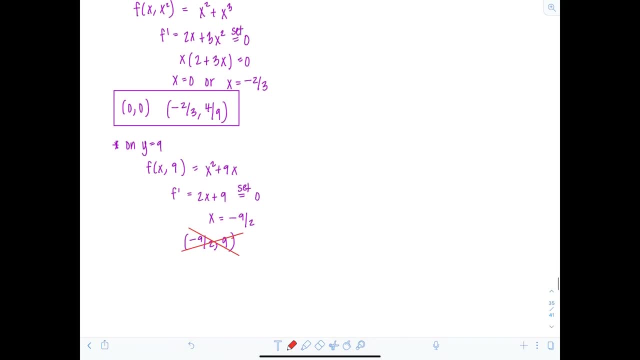 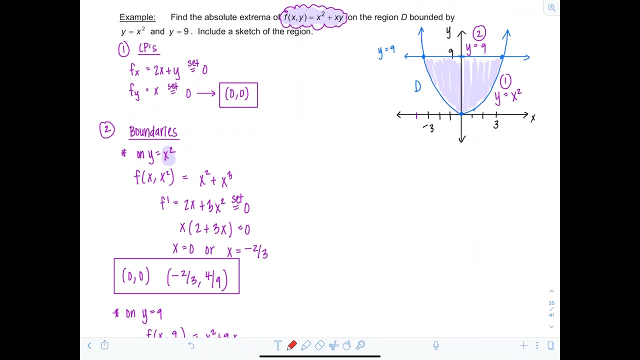 Since it's outside of the region. Okay, The last place that you need to check are the corners, And corners are basically where one boundary equation meets up with another one, So it doesn't necessarily have to look like your typical corner for a rectangular shape. 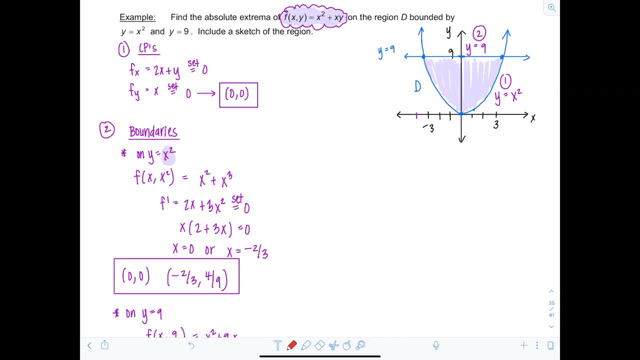 Just anywhere one boundary equation is pasted or connects to another. So I see two corners, don't you? Our corners are right here at 3, 9 and negative 3, 9.. Okay, And then now you're just going to substitute all of these values into the original function. 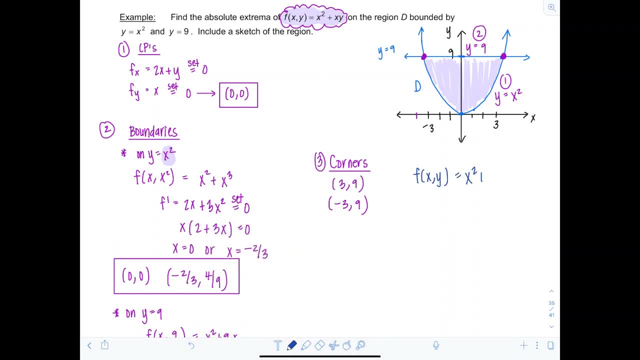 So f of x, y, if you'll remember, is x squared plus x y. So I have how many, How many values to test? We're going to plug in 0, 0.. We're going to plug in negative: 2 thirds, 4, ninths. 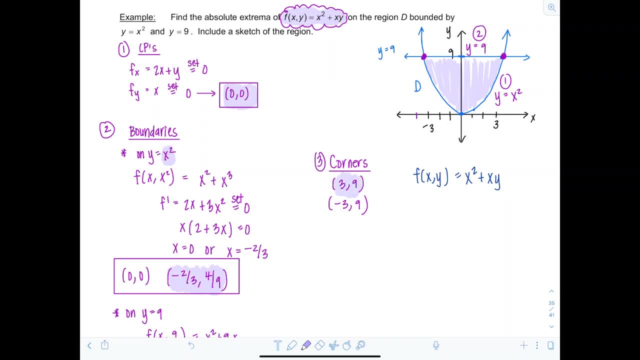 That other 0, 0 is a repeat. And then I have two corners to plug in. So four values. That's not too bad. So f of 0, 0. That's 0.. Not bad f of negative 2 thirds, 4, ninths. 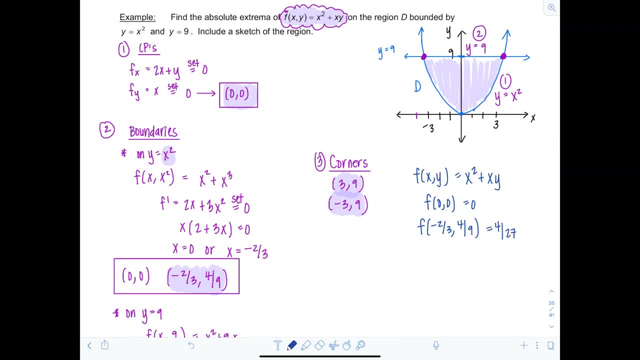 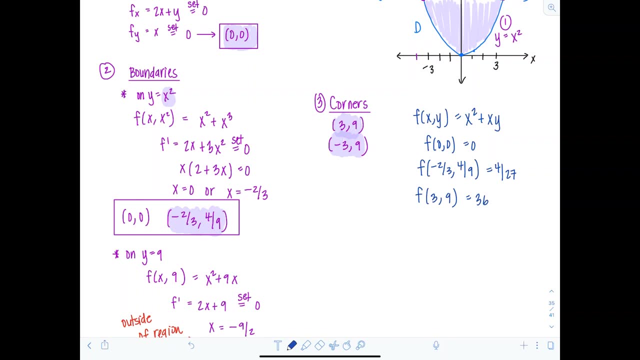 That is 4 over 27.. Woohoo, f of f of 3, 9 is equal to 36.. And f of negative 3, 9 is equal to negative 18.. Okay, So it looks like here is our absolute max. 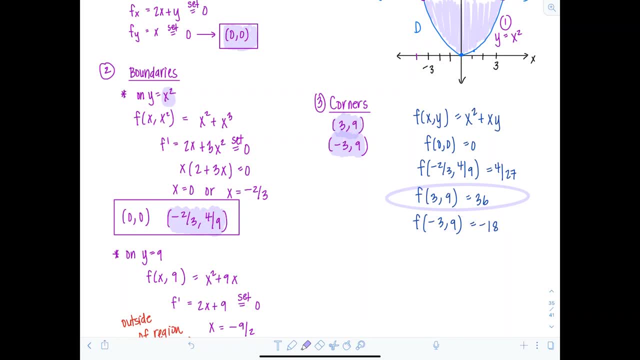 And here's our absolute min: Both of them at the corners. There we go. Okay, So we'll label that now. This was our absolute max, And f of negative 3, 9,, which is equal to negative 18,, is the absolute min. 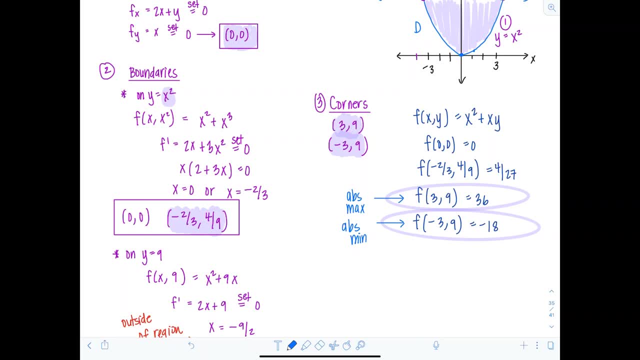 All right, So pretty straightforward process, But just make sure you're working carefully and that you have an accurate diagram of the region D. That way you can identify the boundary properly. Let's move on to a little bit more complicated of an example here. 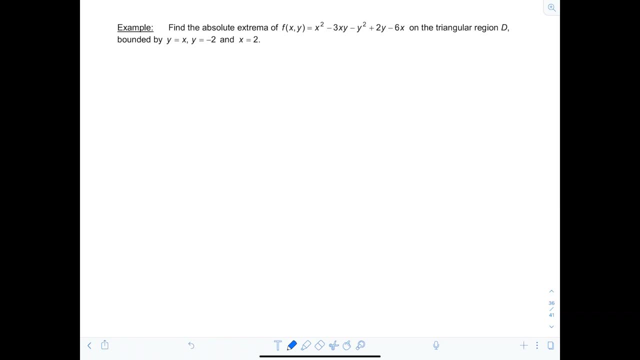 It says: find the absolute extrema. Find the absolute extrema of f of x. y equals x squared minus 3xy minus y, squared plus 2y minus 6x on the triangular region D, And it's bounded by y equals x, y equals negative 2, and x equals 2.. 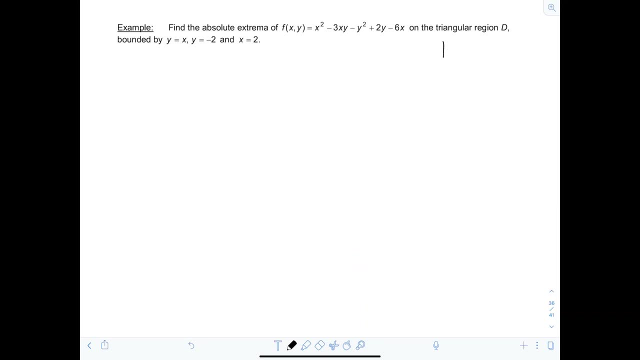 Okay, So let's graph that region first. So y equals x- We know what that looks like, right, And then that's going to intersect: horizontal line y equals negative 2.. And vertical, And then that's going to intersect: vertical line x equals 2, to make a triangle. 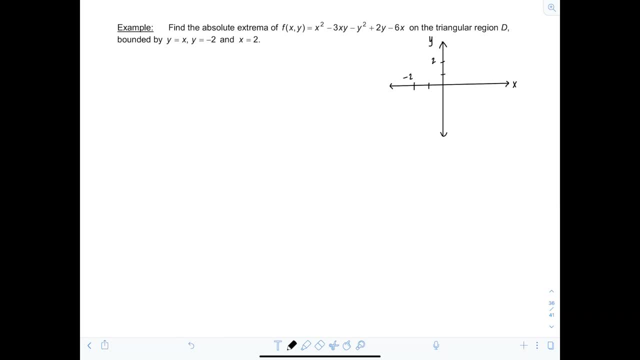 Okay, So there's negative 2, 2, 2, negative 2.. Okay So first I'll draw: y equals x, And then the triangle is formed by bounding that, So that line with y equals negative 2, that's here. 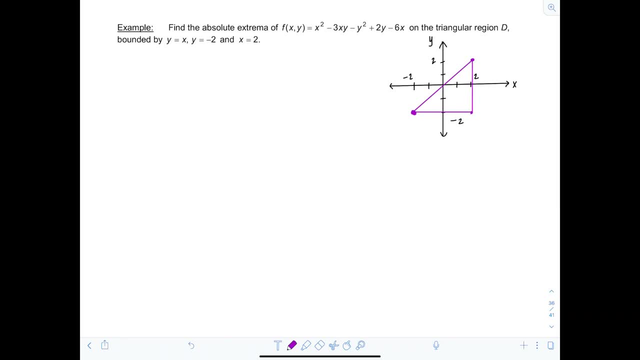 And then x equals positive 2.. So here's our triangle. Okay, I'll label everything in. So notice here: in this case we have three boundaries right. So we have y equals x, We have x equals 2.. And we have y equals negative 2.. 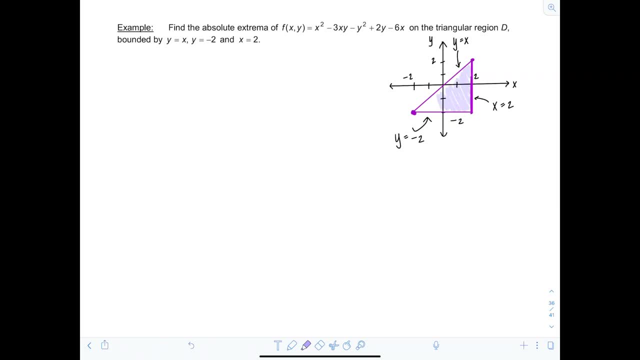 And that's the region D here. All right, Very nice. So start off nice and easy, Just get our critical points. So for critical points, remember we need to take our partial derivatives with respect to x and y. So partial with respect to x is going to be 2x minus 3y. 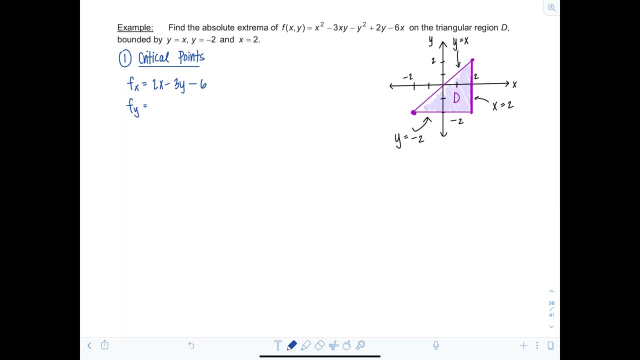 Minus 6.. And then the partial with respect to y is going to be negative: 3x minus 2y plus 2.. And then I set both of these equal to 0.. Since I need them to simultaneously equal 0.. 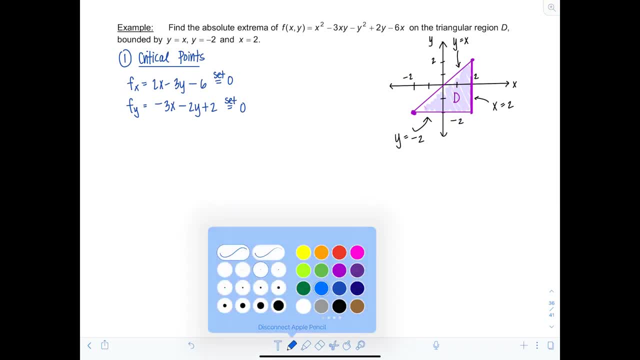 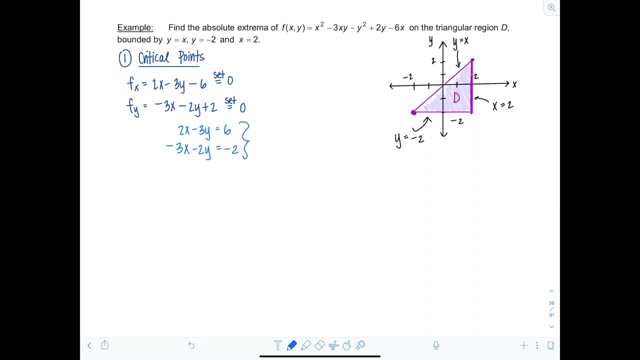 And then I have negative 3x minus 2y equals 6.. And then I have negative 3x minus 2y equals 6.. And then I have negative 3x minus 2y equals 6.. 2y equals negative 2.. So we have to multiply these equations in order for a variable to get. 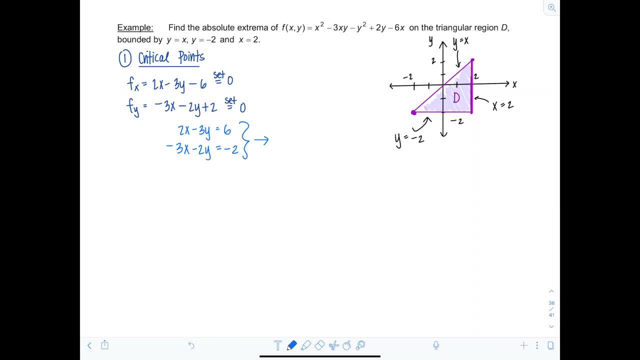 canceled out. Let's try to eliminate x, since it already has opposite signs. So I'll multiply the top equation by 3.. So now I have 6x minus 9y equals 18.. I'll multiply the bottom equation by 2, and now I have negative. 6x minus 4y equals negative 4.. So solving this system, now x is: 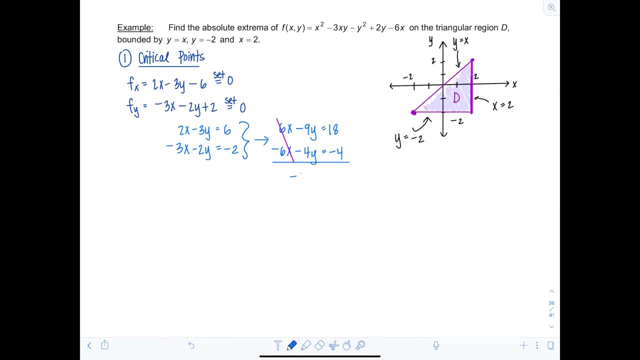 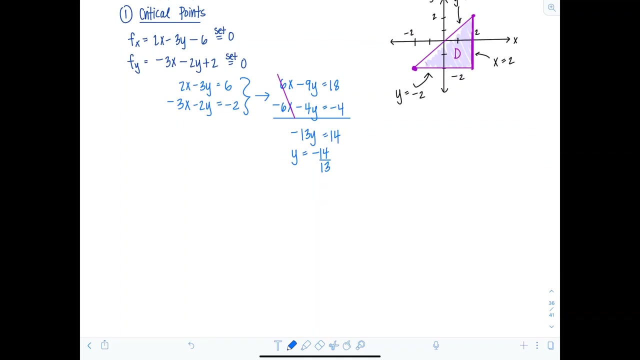 going to cancel out. and then we have negative 13y is equal to 14.. So that means y equals negative 14 over 13.. Okay, not the cutest answer I've ever gotten, but it is what it is. And then we need to. 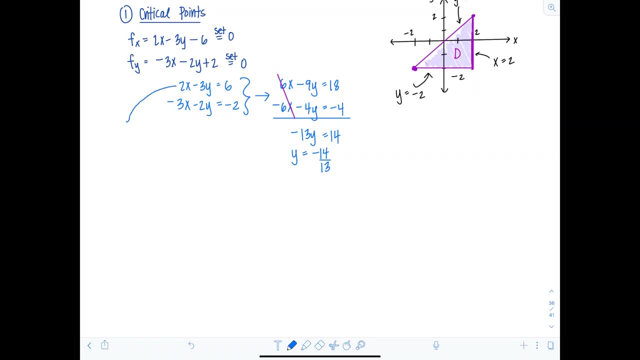 figure out what x is going to be. So let's go back to that first equation: 2x minus 3 times negative, 14 over 13. That's going to give me positive y, 42 over 13,. that equals 6.. And then 6 times 13,, that's going to be 18 plus 60. And then, if I 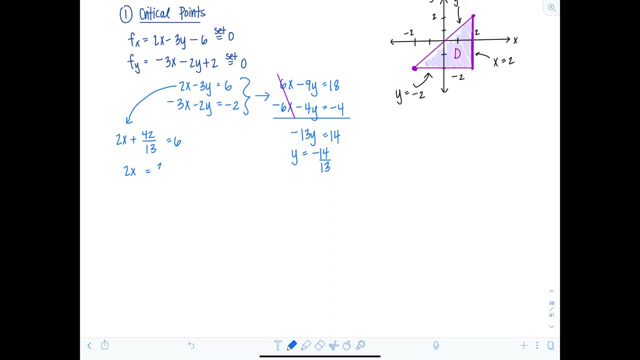 subtract 42, now I'm going to have: 2x equals 36 over 13,, which means that x is equal to 18 over 13.. All right, so we've got a critical point. Here we go. It's 18 over 13. comma negative: 14 over 13.. clicheоне Show Truth. 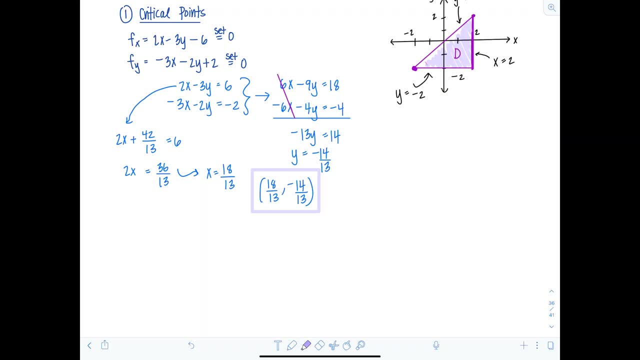 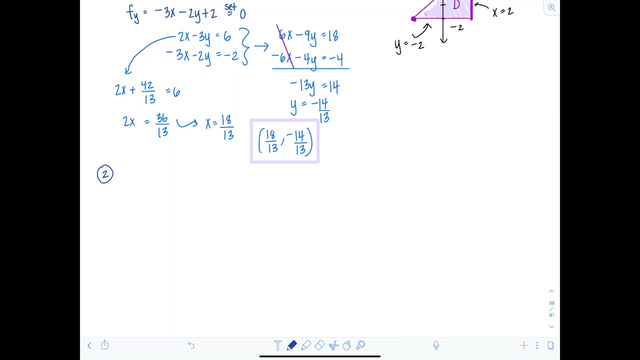 Let's go into the commit function course for 0.. Depth Check. Now, that's the critical point on the interior. What about critical points on the boundaries? Well, I have to check each of the three boundary equations. So Category 2. Boundaries, So I'll 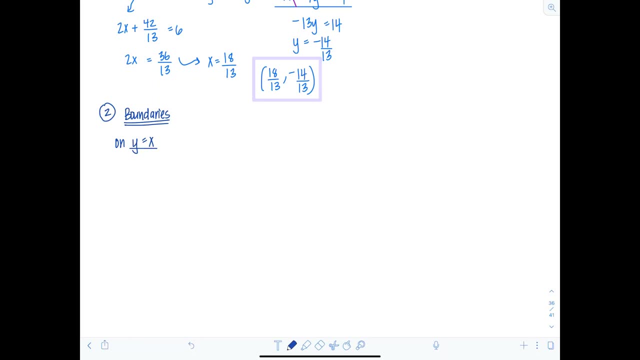 start off checking on: y equals x, 상태 복 remnants: Okay. So on y equals x. I'm going to look at curseكنy Column. So to put that in the going to look at f of xx, substitute in x for y And going back to the original function, this is: 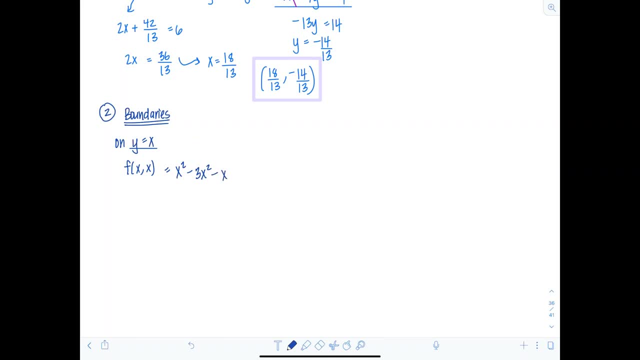 going to give me x squared minus 3x squared minus x squared plus 2x minus 6x. So clean it up. this is going to be negative: 3x squared minus 4x. Now what do I do from here? Remember, you're trying. 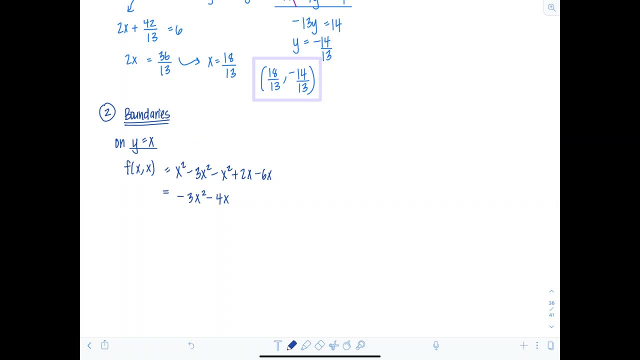 to find critical values, so I need to take a derivative first. So f prime is going to be negative 6x minus 4, and I set this equal to 0, which means that x is going to equal negative 2 thirds. Okay, now what's the y coordinate that would correspond, with x equaling negative 2? 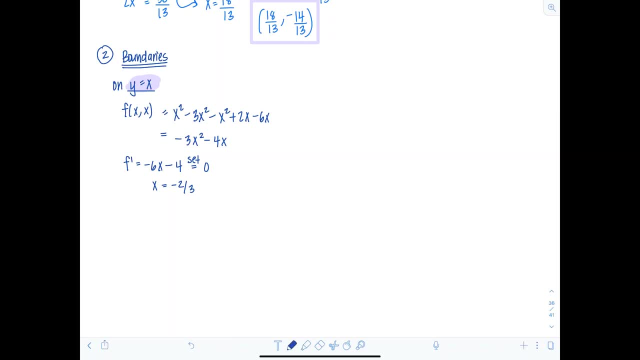 thirds: Remember we got this critical point on the boundary: y equals x. so if x is negative, 2 thirds, so is y. Easy enough. One boundary is done, two to go. Okay, what's the next boundary equation? It is, let's do: y equals negative, 2.. Okay on y equals negative, 2.. So f of x comma negative 2. 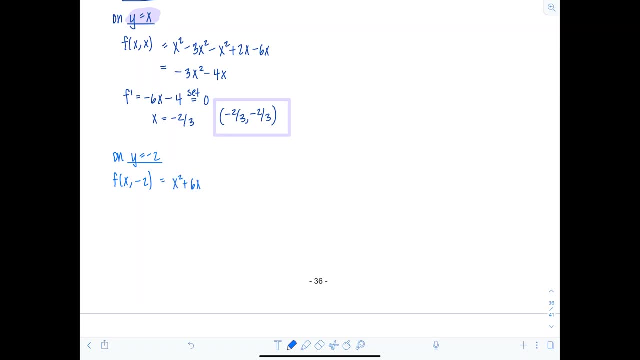 is going to be x squared plus 6x minus 4 minus 4 minus 6x, So I'm going to have x squared minus 8.. Take a derivative, so f prime is going to equal 2x. I set that equal to 0, and I get x equals 0.. 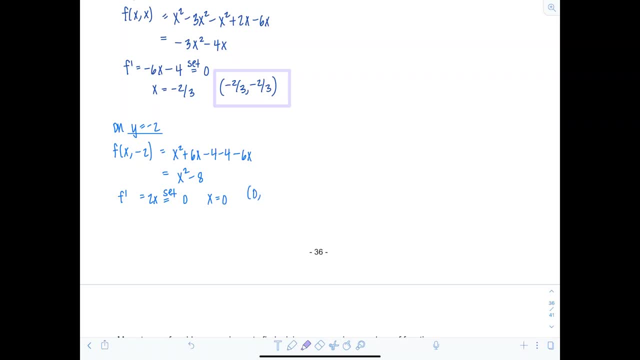 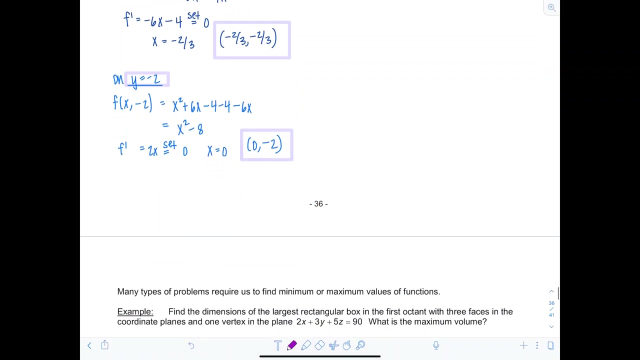 All right. so if x is 0,, what's the y coordinate? Remember, this critical value is on the boundary y equals negative 2, so the y coordinate is negative 2.. All right, one last boundary to test, and that's on: x equals positive 2.. 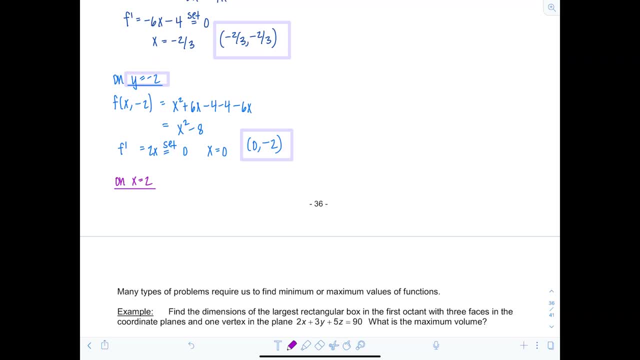 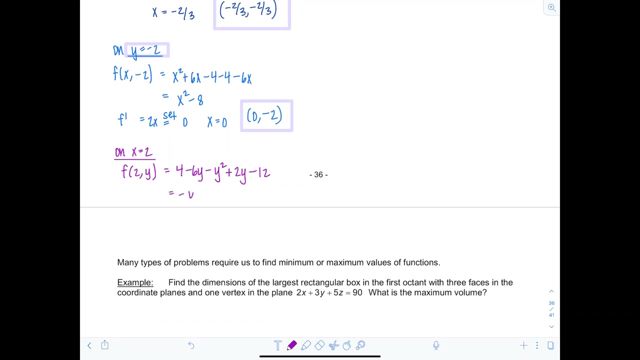 So this one's going to be a little weird, because now I have f of 2 comma y, but don't stress. So then that's 4 minus 6y minus y squared plus 2y minus 12, and you'll get negative y squared. 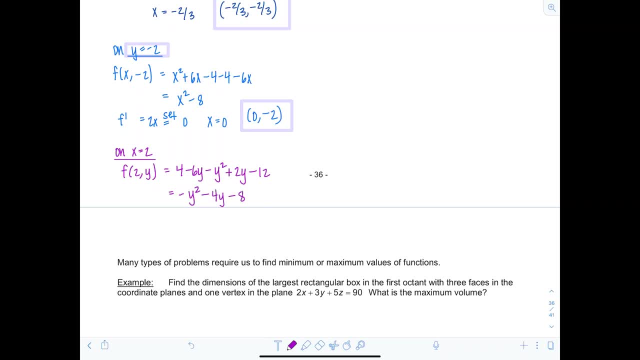 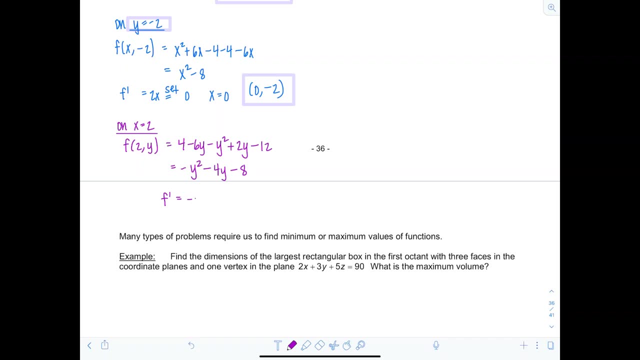 minus 4y minus 8.. What do I do from here? Don't forget this next step. I need to take a derivative. so f prime is going to be negative 2x 2y minus 4.. I set this equal to 0, solve for y and I get y equals negative 2.. 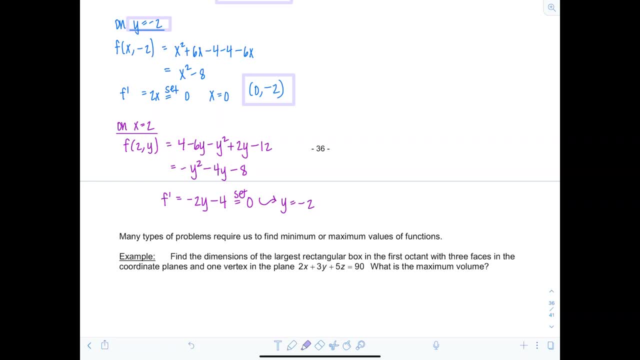 And what's the x coordinate that goes with it? It's positive 2, because this critical point comes from the boundary where x is equal to 2.. So the coordinate is going to be 2 negative 2.. Okay, look at us getting all these potential mins and maxes. 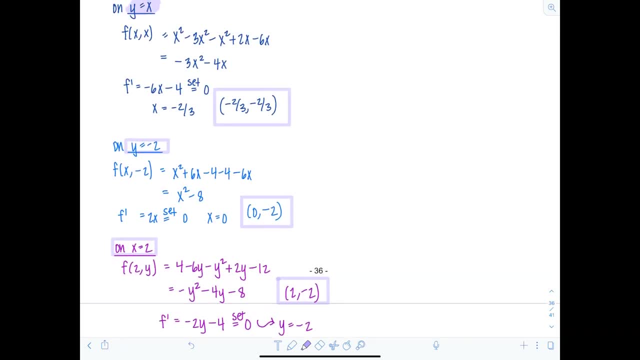 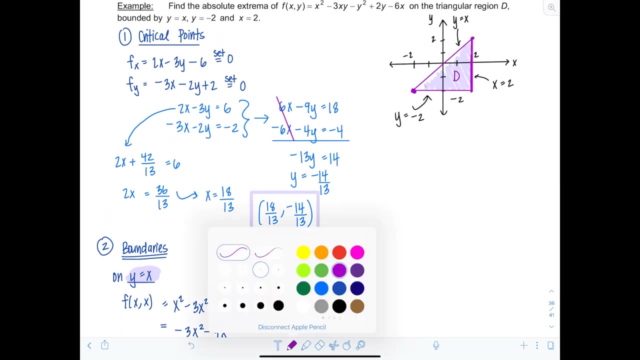 All right. so boundary's done, interior's done. Last thing I need to check are the corners. So look at your picture here. Anytime one boundary equation is pasted onto another one, you have a corner. So I see three of them, don't you? So step three: we've got to list off all the corners. 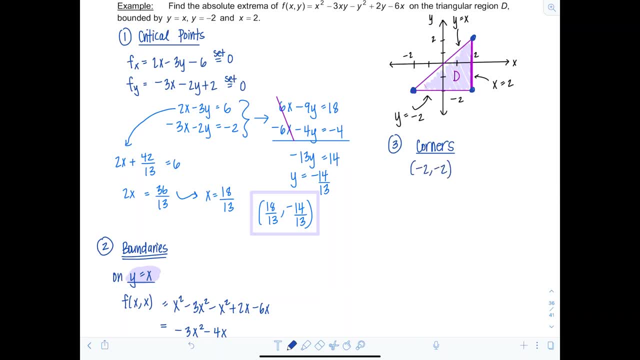 So we've got negative 2, negative 2.. We also have 2, 2.. And then we have 2, negative 2.. Notice this last one here. we actually already got it from the boundary. That'll happen sometimes. 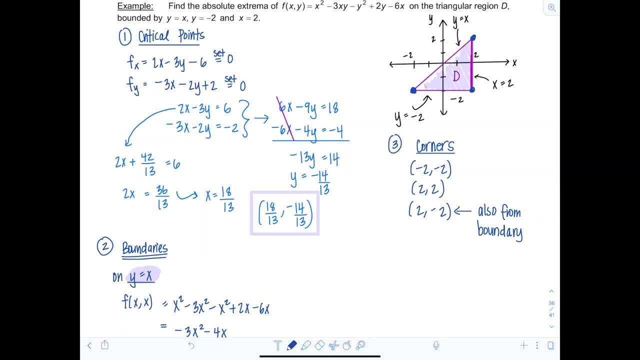 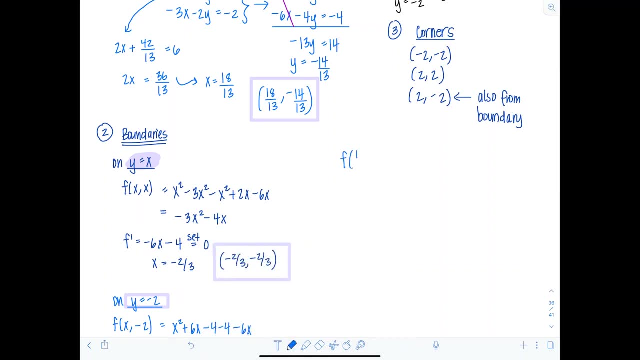 So now let's check all of these in our function so we can identify which one's the absolute min, absolute max value, which one will yield it. So, f of 18 thirds, negative 14 thirds, I mean this should go without saying. but no decimals, people, right Okay? 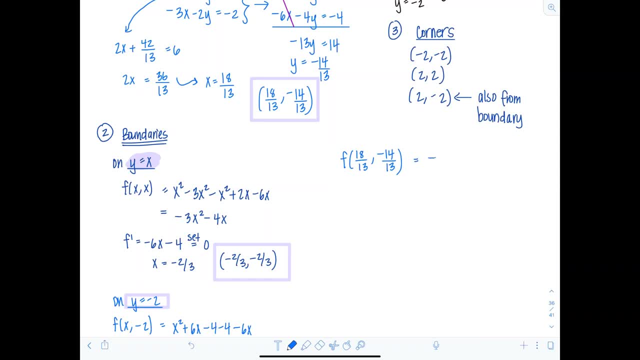 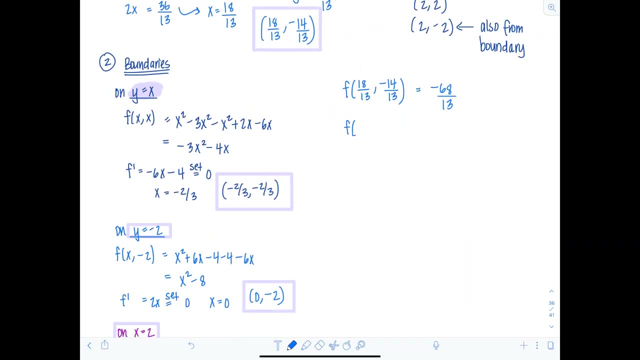 So don't worry, I already did it for you. This comes out to negative 68 over 13.. Then we have f of negative 2 thirds, negative 2 thirds. That comes out to 4 thirds. f of 0, negative 2 is negative 8.. 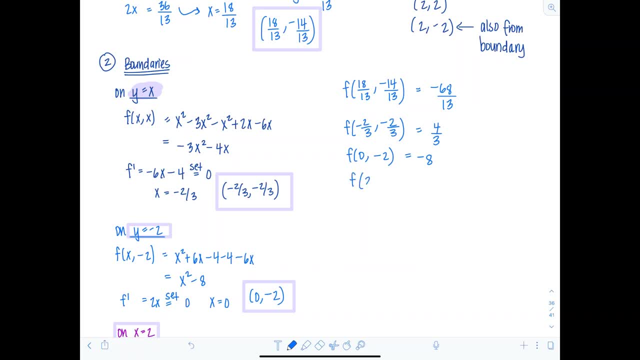 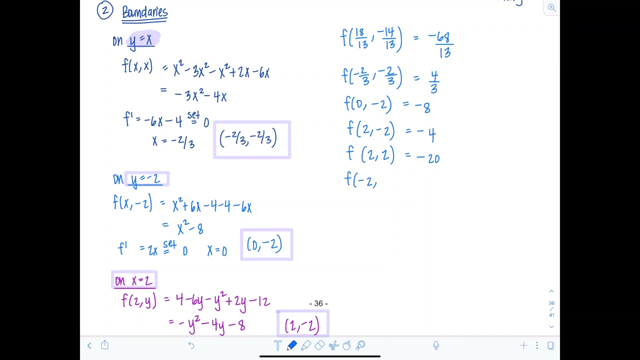 f of 2, negative 2 is negative 4.. f of 2, 2 is negative 20.. And then, lastly, f of negative 2, negative 2 is negative 4.. So let's see here There was only one that was positive, So clearly that's the absolute max. 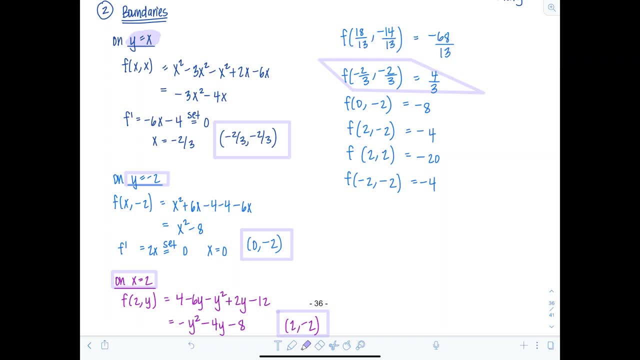 right there. Yeah, whatever shape this is, I like it. And then absolute min is clearly at f of 2, 2,, which is negative 20.. Okay, that's better. Okay, So here is our absolute min And this is our absolute max. 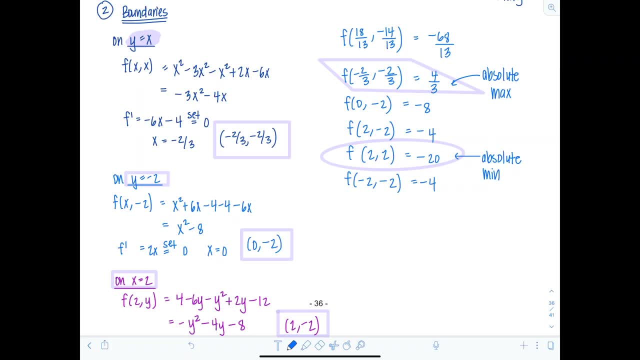 Now they need not be unique, Like if there was another point where I got f of some other x, y, like maybe if I raise this is less than 5,, 6 as a extension, then it'd also be negative 20.. 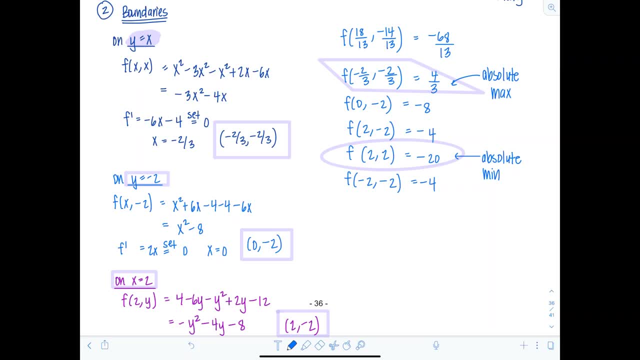 Because if there are all of these points that re gy, Ç, d, then the absolute min value would be negative 20.. But if there are also negative 20, they would both be- the absolute min value would be negative 20, and you would have two points- x, y- that would yield it. 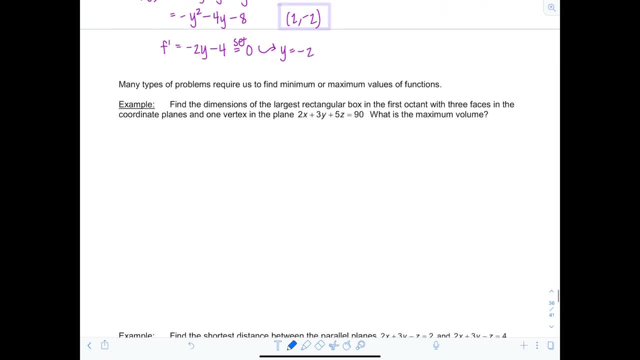 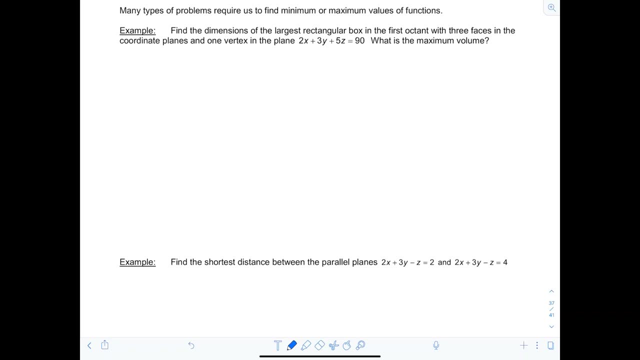 Ok, very good, Now let's look at some applications. Alright, And that's how we'll finish up this little lesson here. So many types of problems require us to find optimization problems and calculus one. So find the dimensions of the largest rectangular box. 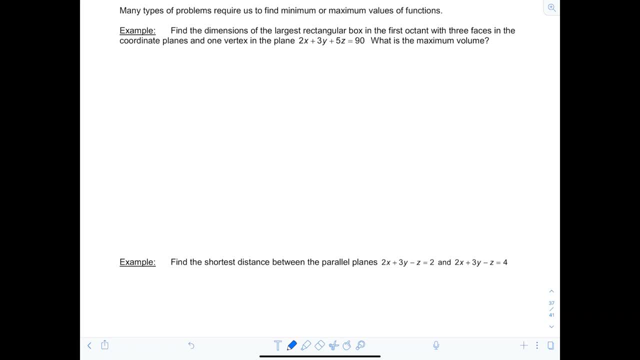 in the first octant, with three faces in the coordinate planes and one vertex is on the plane. 2x plus 3y plus 5z equals 90. What is the maximum volume? So first let me kind of draw out what's going on to help orient things a little bit better. We're making a rectangular box and I'm 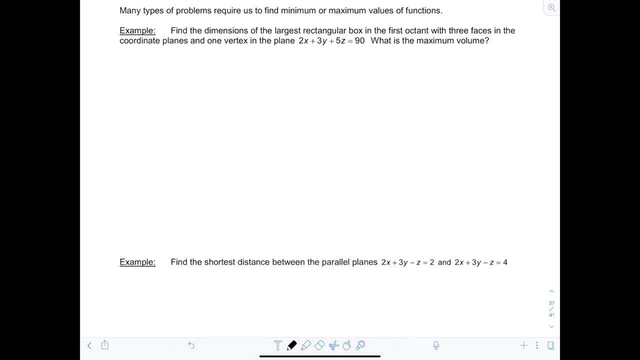 only going to draw the first octant, and the three faces of the box are in the coordinate planes and one vertex is in the plane that's given there. So let's figure out what the intercepts are for that plane so I can draw it out. So let's see here: if x and 1x plus 3y plus 5z equals 90.. So let's see here: if x and 1x plus 3y plus 5z equals 90.. So let's see here: if x and 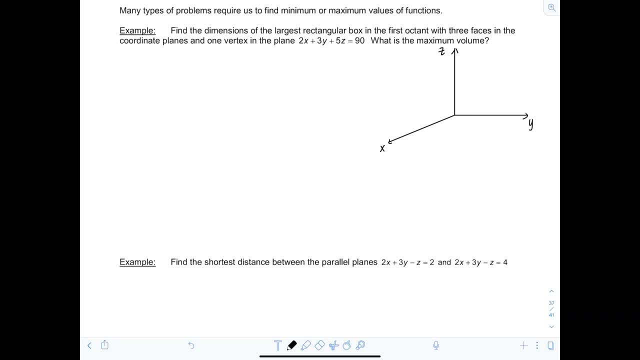 no, let's just say if y and z are 0, x is going to be 45. So here's 45. and then if x and z are 0, y is going to be 30, and then if x and y are 0, z is going to be 18.. So here's this plane in the first. 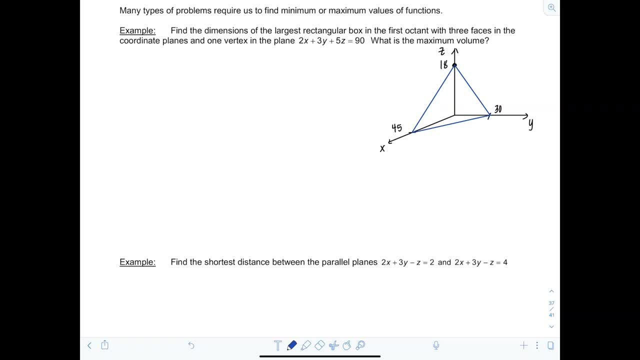 octant, and one of the vertices of the box needs to be touching this plane. So here's the idea. I don't know, maybe the box is somewhere around here and it's going to come out this way. One of the vertices of that box needs to be touching the plane, So let's pretend it's this one, right here. 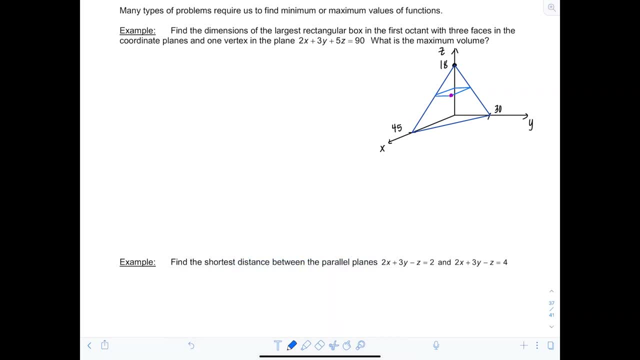 It's touching the plane Comes down like: so All of the faces are in the coordinate planes. Okay, well, I could move that point. I could lower it and have maybe a wider box, or raise it skinny or taller box, I don't know. What I want to do is maximize the volume of that box. Okay, well, how could I find the? 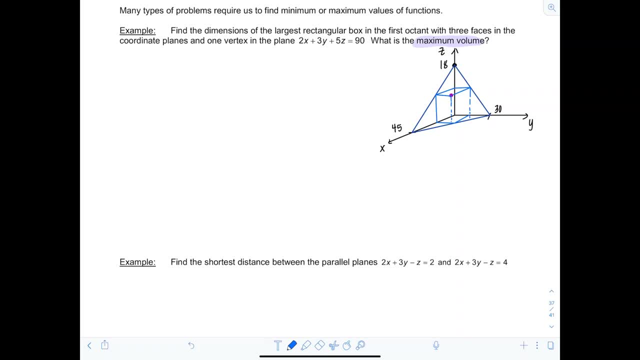 volume of the box. Well, it's really all determined by that coordinate that hits the plane, because the volume would be given by x times y times z. right, because those are the coordinates right there at that point: x, y, z, that's on the plane, right here, given by this equation, and x would give me the length, y would 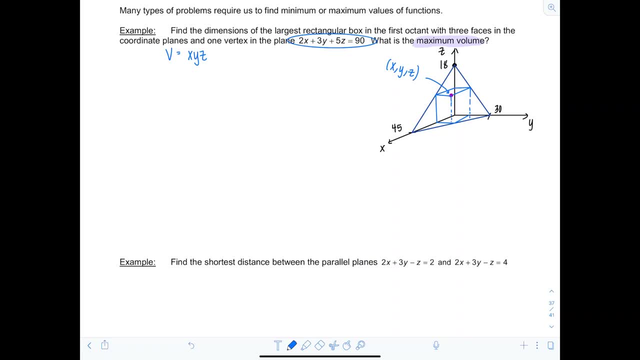 give me the width and z would give me the height. Okay, well, I want to write this as a function of two variables. that way I could find where this max volume would occur. So why don't we solve for z in terms of x and y? We can do that easily. So z is going to be one-fifth times 90 minus 2x minus. 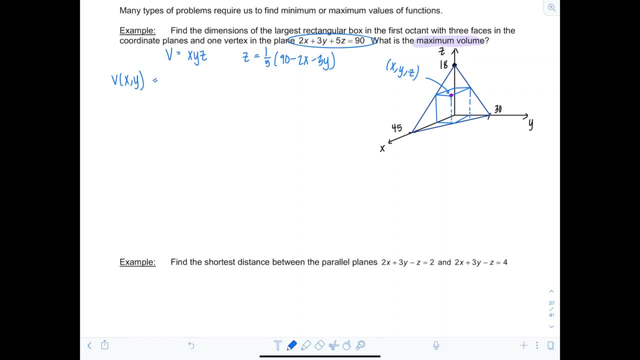 3y, and so now I can write v as a function of just x and y and I have one-fifth x- y times 90 minus 2x minus 3y. Okay, let's distribute a little more, So v of x- y is going to be one-fifth times 90 x- y. 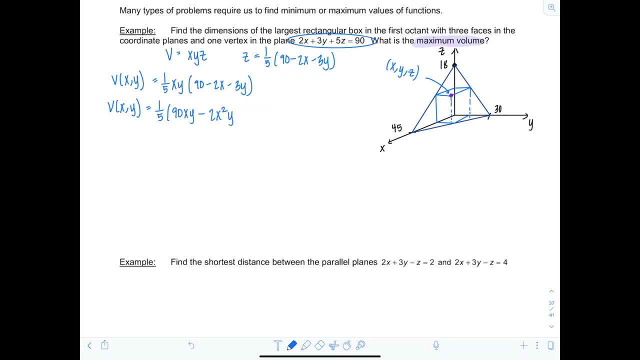 minus 2x squared. y minus 3xy squared. Now I'm ready to go take some partial derivatives so we can get critical points. So partial with respect to x, just leave that one-fifth, and then now I'm going to treat y as a constant. so I'm 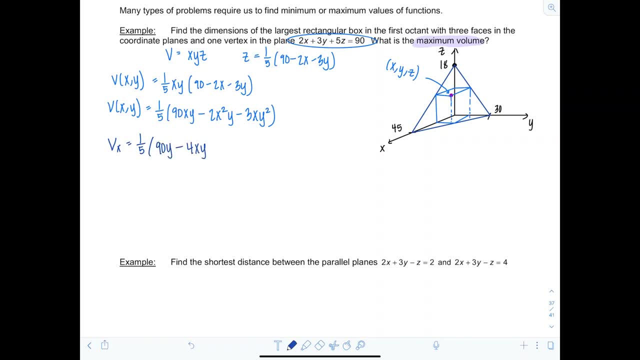 going to have 90 y minus 4xy minus 3y squared. And then I'm noticing here I can factor out a y from everything. so this equals one-fifth times y times 90 minus 4x minus 3y, And I want to set this equal to zero. 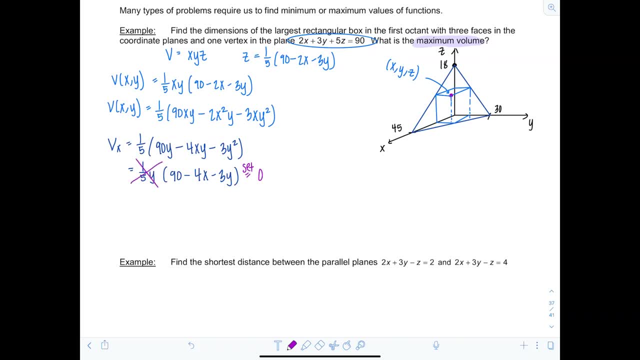 And, interestingly, I'm going to throw away the case where one-fifth y is zero, because then the volume would be zero, right, and I'm trying to maximize the volume, So that's not going to be interesting to me. only this condition here. Now let's repeat the process, Let's take the partial, with respect. 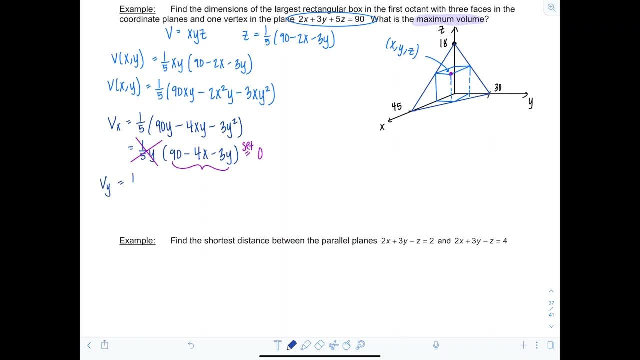 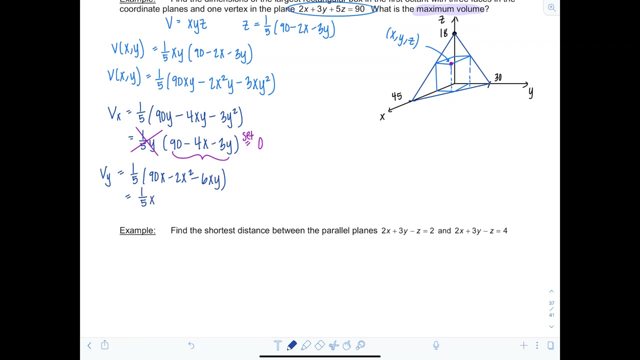 to y. So partial with respect to y is going to be one-fifth 90x minus 3y. So I'm going to take that x from all of the terms again. So I have one-fifth x times 90 minus 2x. 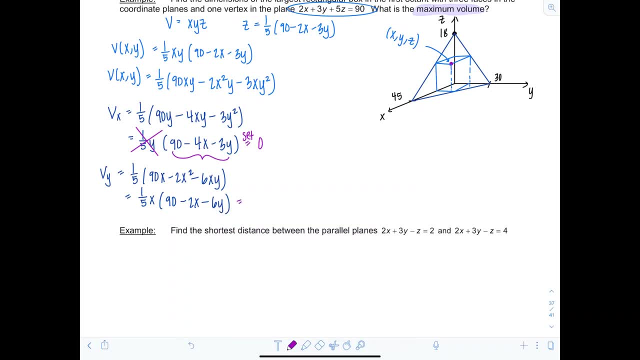 minus 6y, And again I'm going to set this equal to zero And I'm not interested in one-fifth x equaling zero. right, x can't equal zero, y can't equal zero because we're doing an application problem And if I'm trying to maximize volume, it doesn't make sense for me to have 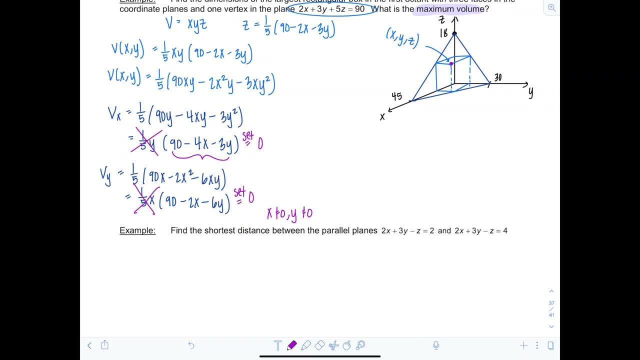 either of the dimensions being zero. So now I'm going to solve this system here where 4x plus 3y is equal to 90.. That comes from here, Setting this equal to zero. And then you know what? Let's get this show on the road. I'm going to multiply this equation through: 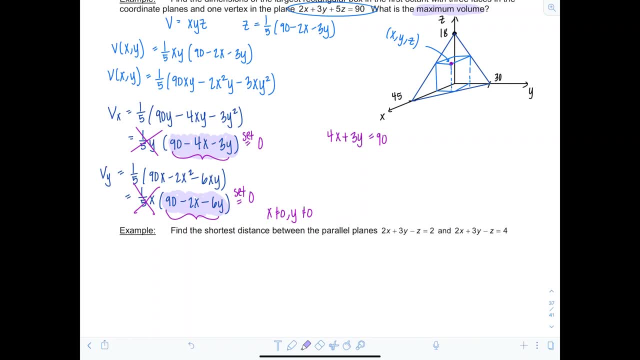 by a negative 2 and move that 90 over. So now I'm going to have negative 4x minus a 12y equals negative 180.. Okay, so now my x's are going to cancel out And I have negative 9y equals negative 90, which means y is equal to 10.. 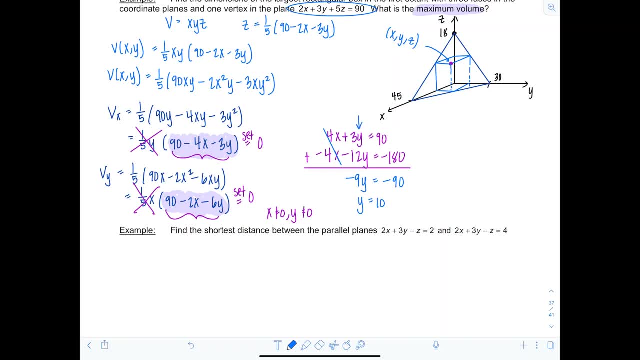 Okay, cool. So if y is 10, you can just substitute that back in there. That's going to be 30.. So that means 4x is equal to 60.. So x would be 15.. And then we can do this again. So we have negative 9y equals negative 90. 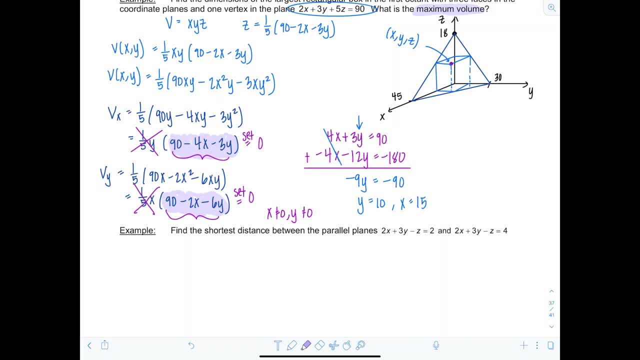 And then we can just come back to the equation of our plane right here. And if I know x is 15 and y is 10, then that means z needs to be 6.. Okay, so that those dimensions that point on the plane. if one of the vertices of the box is at that point, it will yield the max volume. 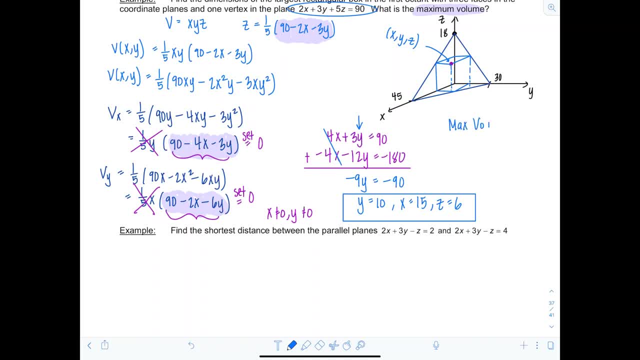 And what is the max volume? Well, it's just the product of those three numbers. So the max volume is going to equal 15 times 6 times 10, which is 900.. They didn't give me any units, I'll just put units cubed, so I. 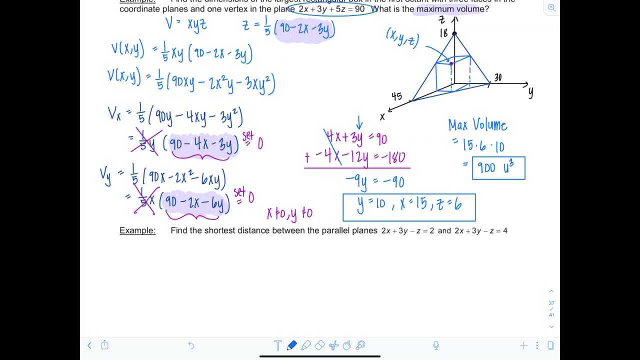 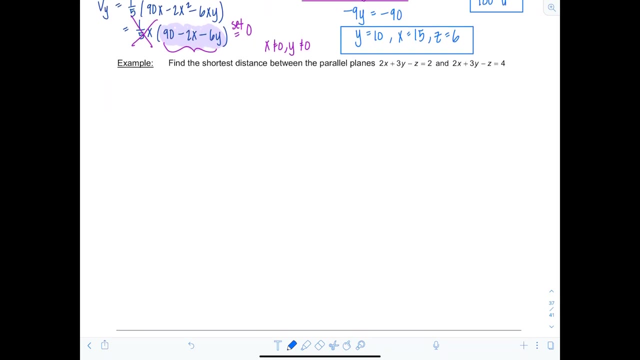 feel good about it: 900 units cubed. All right, very good. One last example, and then we are done. So find the shortest distance between the parallel planes. 2x plus 3y minus z equals 2.. And 2x plus 3y minus z equals 4.. Okay, we have another way to do this right that we studied. 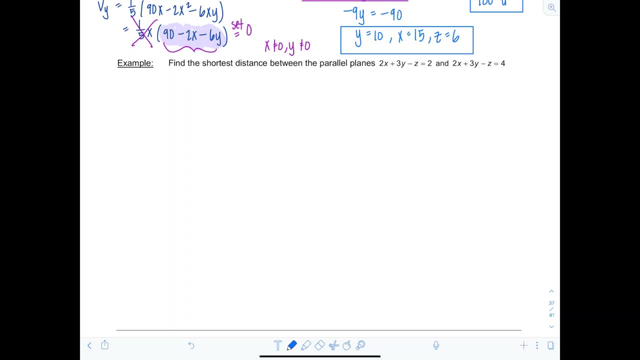 in a previous lesson dealing when we just focused with planes and lines and things like that. But I want to use the new methods that I have, So what we're going to do is take a point from one plane and connect it to an arbitrary point on the other plane. What do I mean? Okay, so can you. 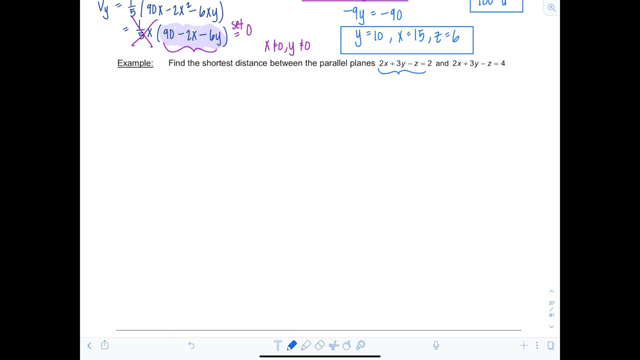 easily find a point that's equal to 2x plus 3y minus z equals 4.. And 2x plus 3y minus z equals 4.. I'm going to use 0,, 0, negative 2.. Right, and these planes are parallel. so look, this is what's going on. 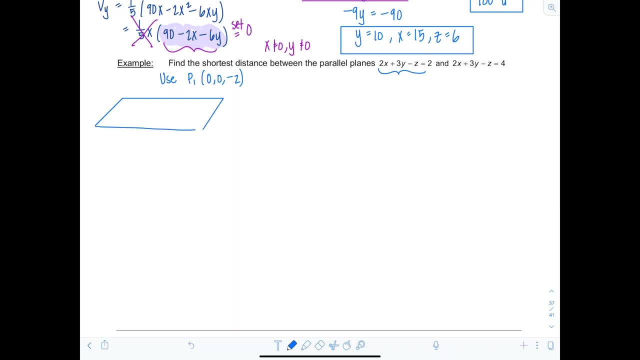 I thought this is why I can pick any point, because they're parallel. So here's plane one, and then I'll copy it. Here's plane two, And I want to know what the distance is. So I'm going to pick 0, 0, negative 2.. 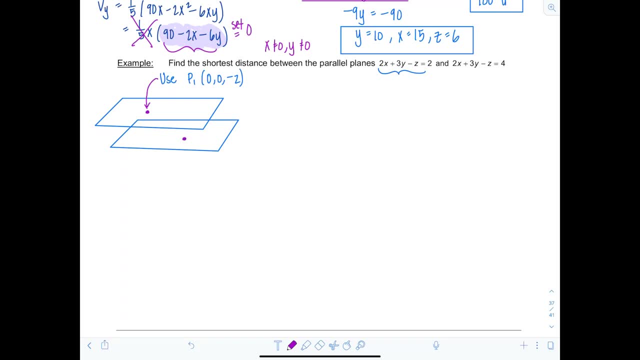 And I'm going to connect it to some arbitrary other point on this plane here- x, y, z- And then this is going to be a function. I'm going to try to minimize it and then eventually it once I find the minimum that's going to give me the shortest distance between the two planes. 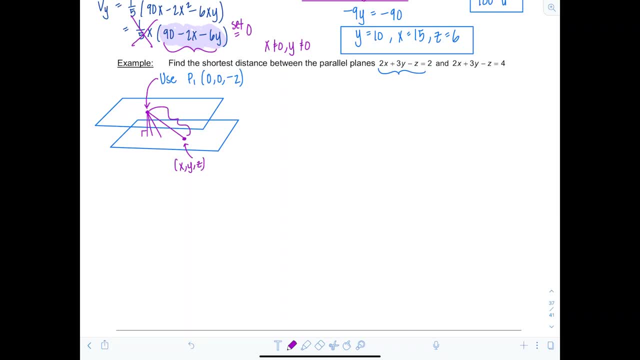 Okay. so how do I say to some arbitrary point on the other plane, Well, I want to connect it to p2 with coordinates x, y and then instead of z, let's rearrange here. I know z is going to equal 2x plus 3y minus 4.. So that's what I'll have here: 2x plus 3y. 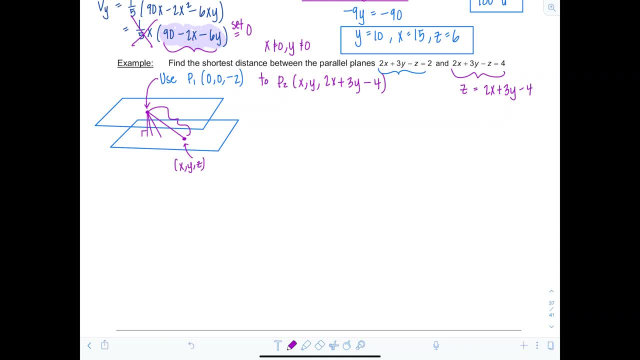 minus 4.. Okay, do we have a formula to find the distance between these two points? Absolutely, but it involves a square root. So common practice is: instead, we're going to minimize that matrix by taking the distance squared, which I'll call f, because it needs to be something odd. So I'll continue the symmetric calculation. 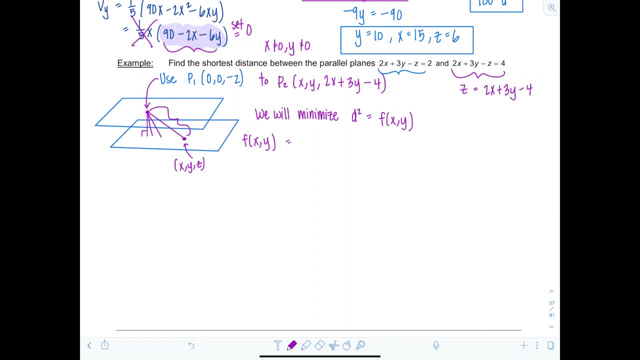 And the minimum that I've wanted to have is now the distance squared, which I'll call f, of x, y. Why do I do that? Well, the minimum will still be achieved at the same, talvez x and y. It's just going to be an easier function to work with. 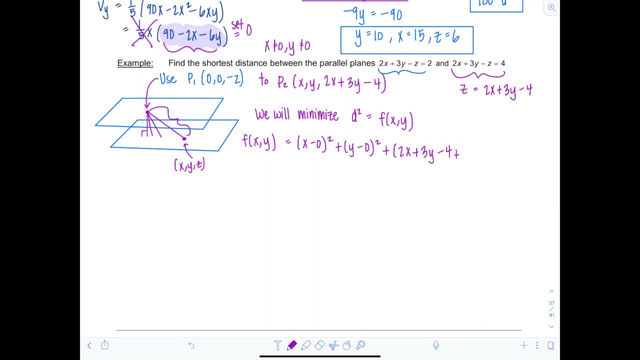 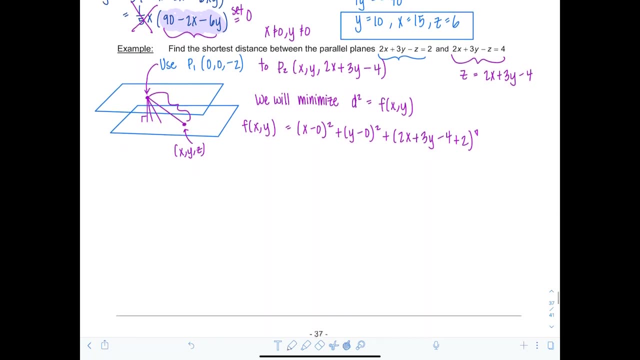 Okay, so f of x, y, four plus two squared. See, aren't you glad you don't have a big old square root outside of all of this? I sure am. And then now let's go ahead. let's take our partial derivatives, Shall we? 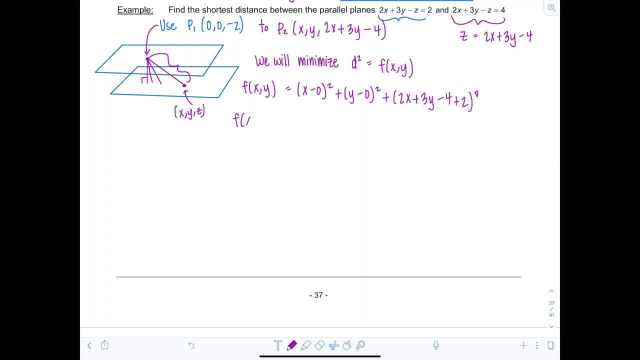 clean up a little bit more. Yeah, let's do that. So f of x- y equals x squared plus y squared plus that should be a two, Two x plus three, y minus two squared. And for goodness sake, don't multiply this out. I mean, that's why we learned the chain rule right. So partial with respect to x is going. 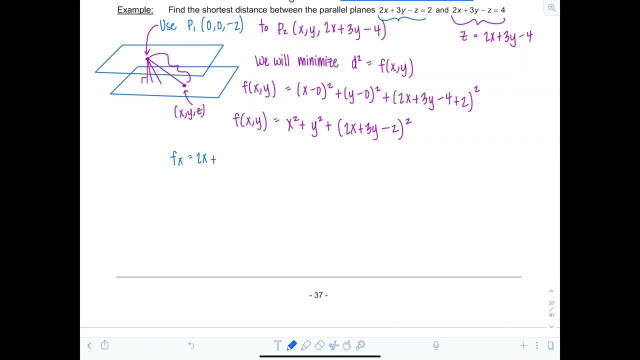 to be two x plus. I'm going to have to bring this two down And then, when I apply the chain rule, I'm going to multiply by the derivative of the inside with respect to x, which is two again. So I've got four times two x plus three. 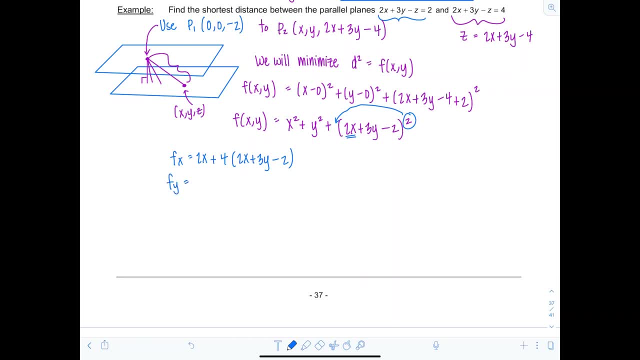 Y minus two, And then partial with respect to y is going to be two, y plus six times two, x plus three, y minus two. I'm going to set both of these equal to zero. Oh, it looks nice. They're just both linear equations. I love it. So here, distributing the four and then combining like terms, we're